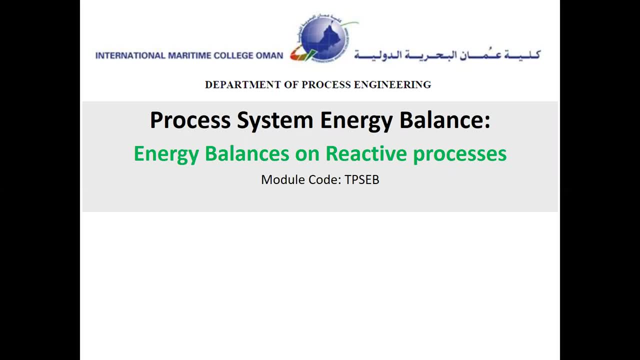 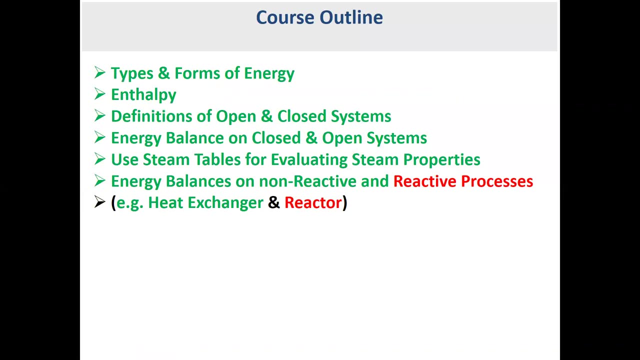 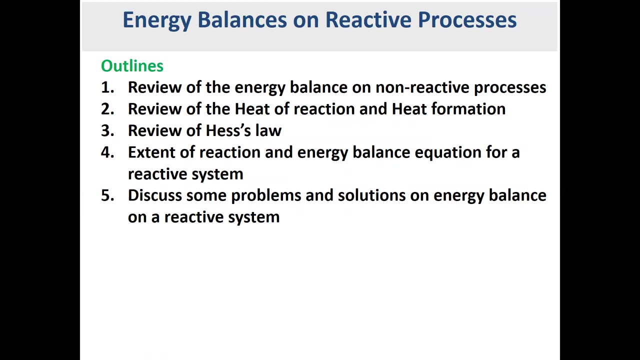 I uploaded on Moodle and come back to me anytime if you have any question or any doubt. So by actually knowing the course outline, I will review what we want to study in this video and this week of the study. So first of all, I will review for you the energy balance. 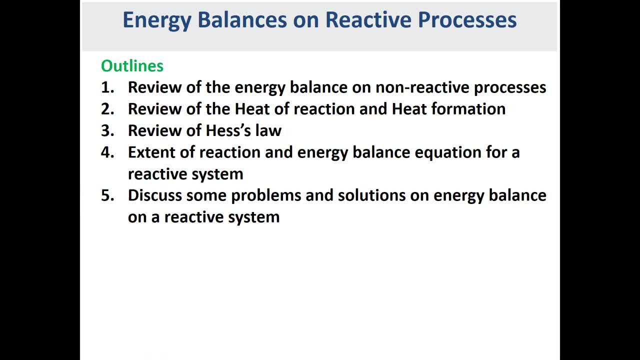 on nonreactive processes that we did in the third week of the study, Just for you to remember, because you need this part for this chapter, And then we will actually study the Moodle, actually a study together. some general point and introduction, introductory part of the this chapter 9 about reaction and reactive processes. then we review the. 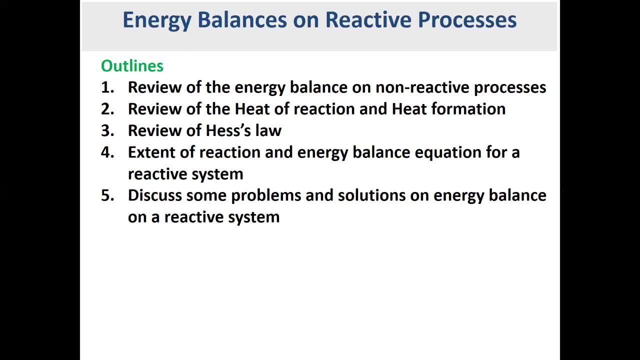 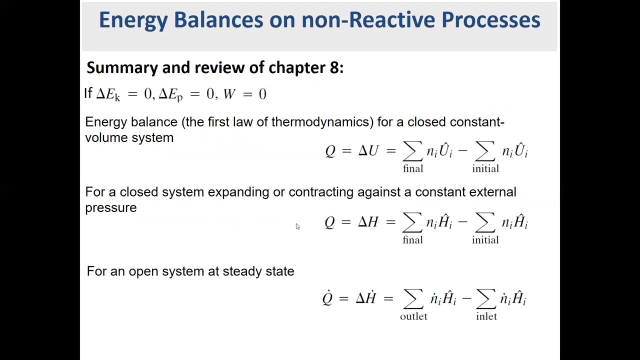 Hess law and we come back actually to some terminology of the chapters and finally we will study more with some problems and showing you the solutions of those processes when there is a reactive process. so if you go back to chapter 8, we learn if we have a process that there is low values or negligible. 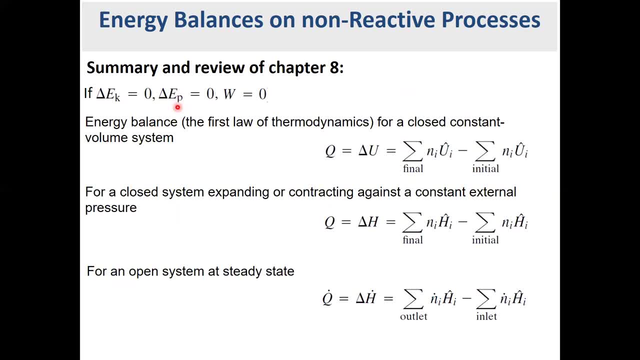 values of the kinetic energy and potential energy or there is no kinetic energy, potential energy changes in the process. while there is no work energy transfer in form of a work, we can reduce the energy balance equation to Q to heat equal to changes of internal energy for a closest, the closed constant volume. 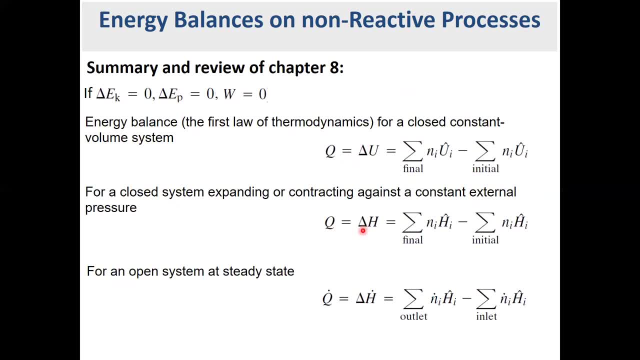 system. and to Q, equal to changes of internal energy for a closed system expanding or contracting against a constant external pressure. and finally, for it is written, the rate of heat transfer is equal to the changes of the rate of enthalpy transfer into LP changes for an open system at the steady state condition. so I provide 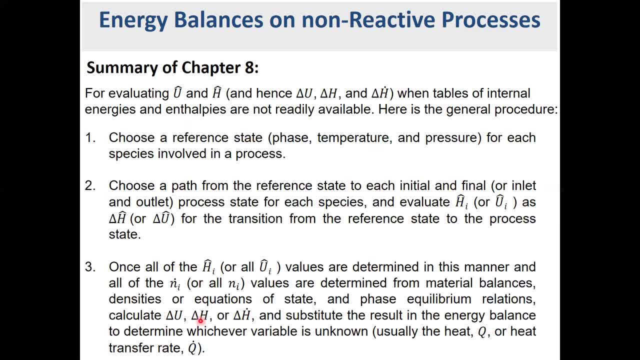 it for you the steps that you have to consider to solve or to actually to do the balance of energy on non-reactive processes. so we learn that if you want to calculate the internal energy, a specific internal energy or a specific in toll P, when there is no table with ready available data, so we have to do. 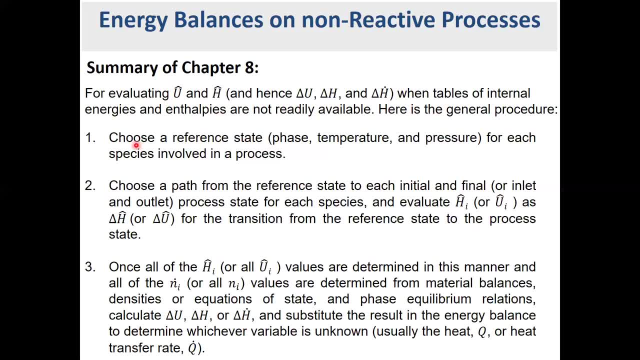 some steps to provide and calculate these values. so I told you you have to select the reference state first. this reference state should be: should has a known phase, temperature and pressure for each species involved in that process. then we construct the path from the reference state to final state of the that component in the process and we evaluate. 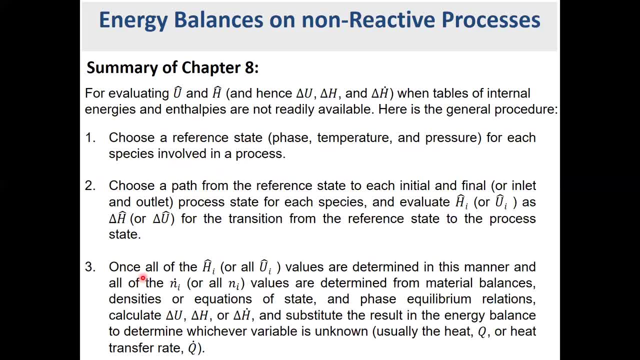 the transition in each steps. so, as you know all the values and, if you remember, we provided an inlet-outlet enthalpy table, so we put all the data of the mole rate and specific enthalpy rate and then it was easy for us to calculate all. 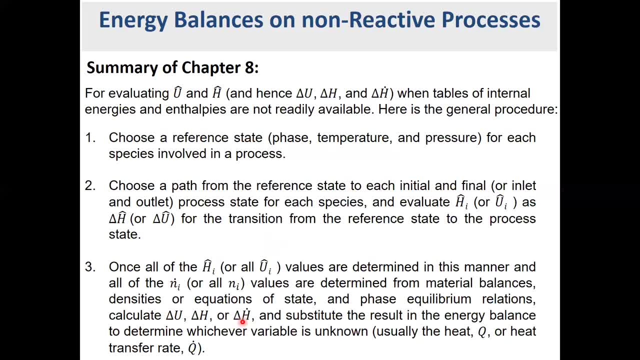 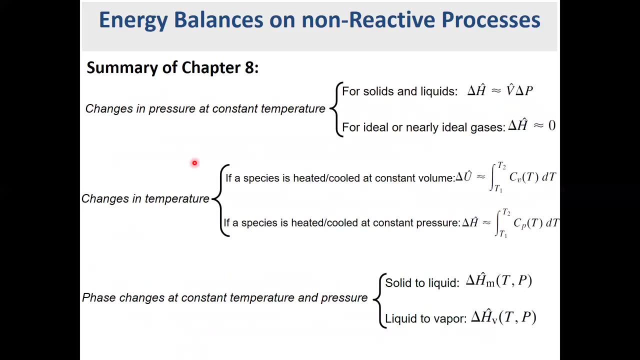 the delta H or actually delta U changes through using that table. and finally, we can substitute the values of delta H in energy balance form and calculate heat or heat rate or transfer rate, so to be able to calculate the enthalpy changes on the from the reference. 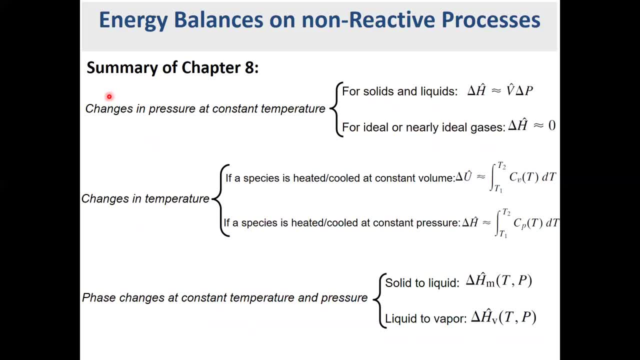 state to the final state. in the process, I show you how to calculate by using the changes of pressure, changes of temperature and changes of phase transition. so, if you remember me, we actually I asked you to use either to to actually change either temperature or pressure or phase at once. if you want to construct the path, 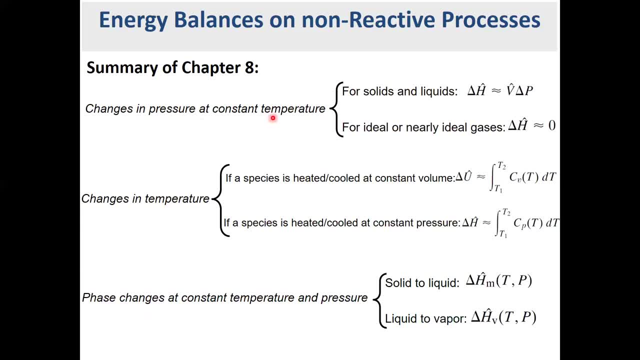 so if there is changes of pressure at constant temperature and for sure that there is no changes of the phase, you can. if it is solid and liquid, the changes of the entropy will be equal to v, cap, delta, p or a specific volume multiplied by changes of pressure. and if your component is ideal, 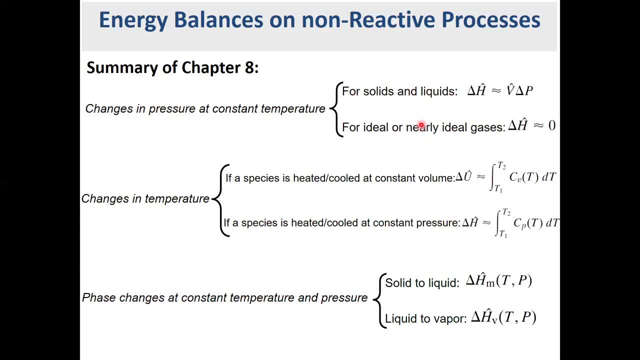 gas, or nearly ideal gas, or with the gas with very uh, low pressure to like some atmosphere. you can consider. you can actually neglect the amount, the changes of the intel for process with changes of temperature. if it is at constant volume, you can use this equation, while if it is in the constant 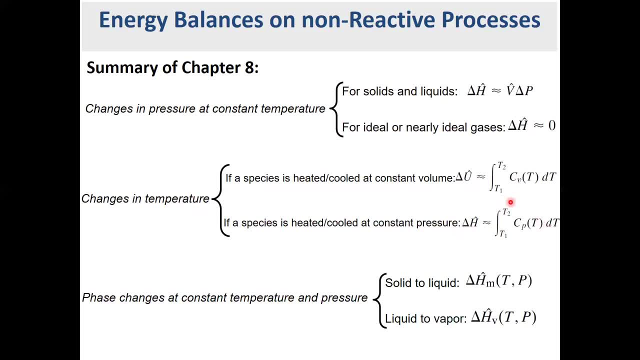 pressure. you can use this equation to calculate that changes of enthalpy at con, at constant pressure and pressure and temperature change. and finally, if there was any phase change, while there was no temperature change, no pressure change. if there was conversion between solid and liquid, you have to use fusion heat and if there is changes between liquid and vapor means liquid. 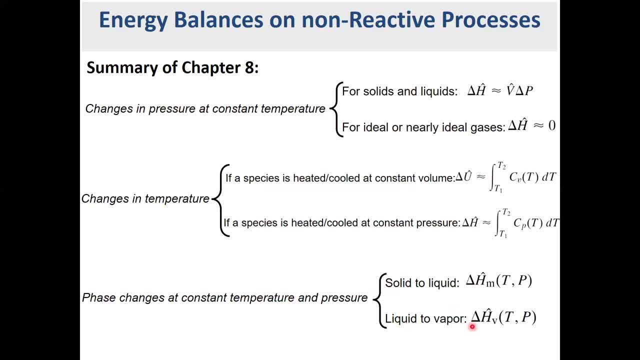 to vapor or vapor to liquid conversion. you have to use evaporation heat for sure. if the heat is positive, it is liquid to solid to liquid and is negative if if actually there is the other way. i mean i don't mean negative or positive of the values, i mean 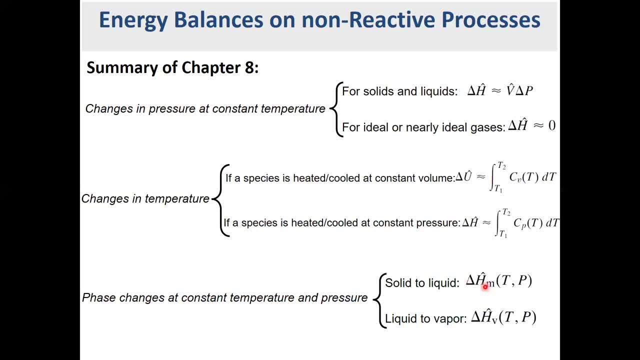 negative or reverse form of what you see in the table or what you have as the delta hm or delta hm. so um for uh, in, actually in your textbook you have delta hm value and delta hrv value in table b1. as i show you in the previous session that, however, these values, that is provided in table b1 is only. 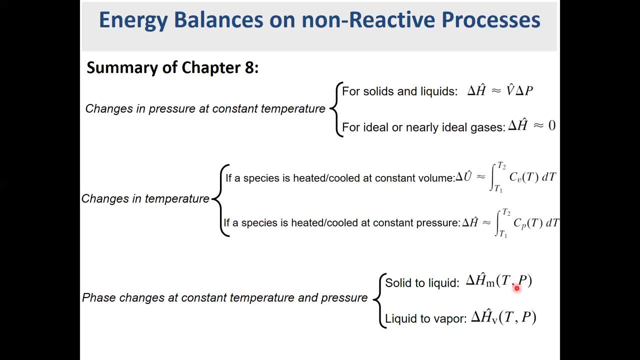 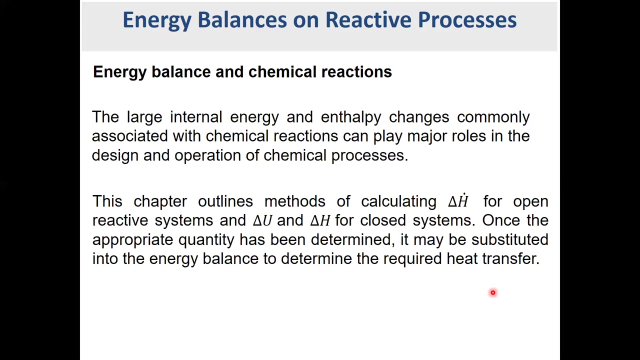 for uh at 25 degree and one atmosphere pressure and it's not uh. you cannot use them for other temperature and pressure. so this is what we learned so far and i hope you can actually just remember what we studied in the third week of study. so today we want to focus most on the reactive processes. when you have a 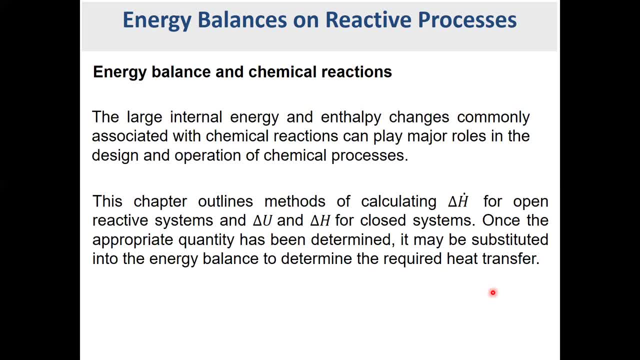 reaction involved in your process. first of all, you have to understand that the amount of internal energy and in tall p, associated with chemical reaction are quite huge and large and they are playing a major role in design and operation of chemical processes. so we have to, we have to consider how to calculate them to be able to 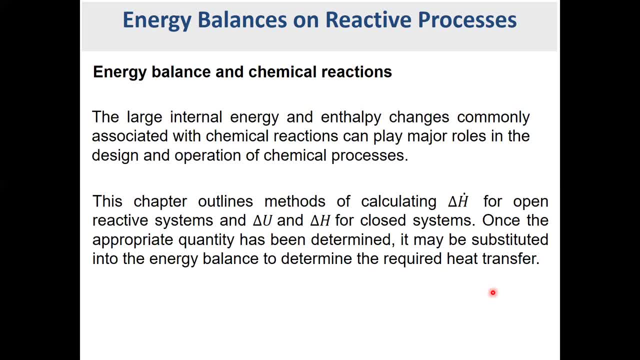 do the energy balance on reactive processes. in this chapter we learn how to calculate delta h, or actually for delta h i mean changes of intel p rate for open system or delta u and delta h for closed system. so once we have these values, as you know, we have the value, so we can easily 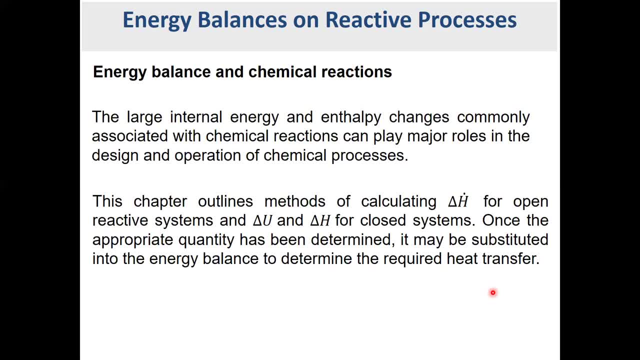 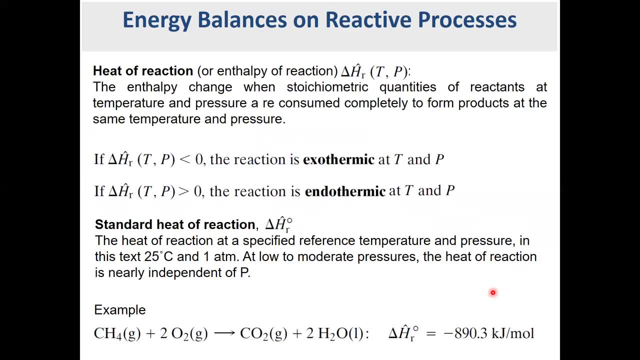 can refer to the energy balance equation or first law of thermodynamics and calculate other parts of the equation, like, for example, if it is heat, so we can calculate as we discussed. so before that, I want to give you some definition of different point, like introduction part of this chapter, so we will go through. 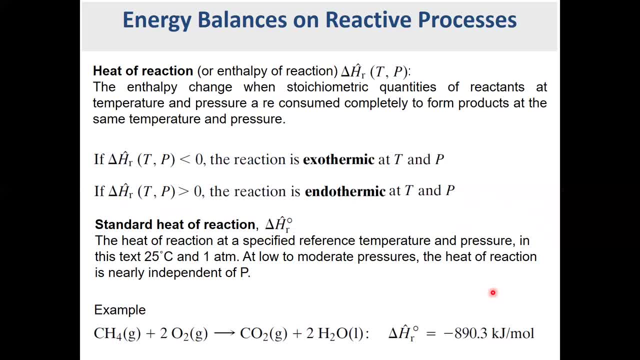 some, some actually general points to be able to understand final calculations. so first of all, I want you know what is a heat-up reaction. heat-up reaction is the enthalpy change when sto- stoichiometric quantities of reactants at temperature and pressure are consumed completely to form product at the same temperature and 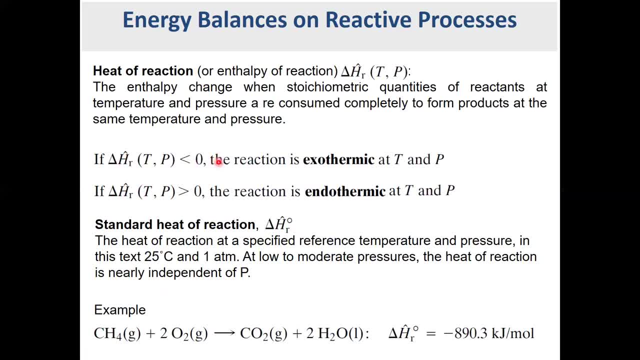 pressure. so if the value is negative, the reaction is exothermic and if the value is positive, it is endothermic. I want you go to the book and a study about these two term to understand what does it mean, or remember, just because I'm sure you already know what does it. 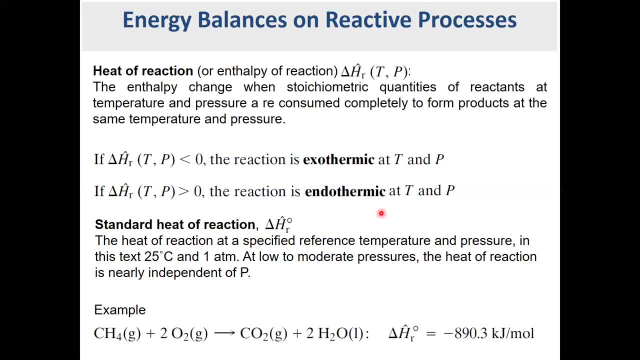 mean? just to remember, what does it mean exothermic? just for your own review: if the process or reaction is exothermic and the HR is negative, it means that less energy is required to break the bond holding the reactant compared to the energy you need to break the to form the products. so means in. 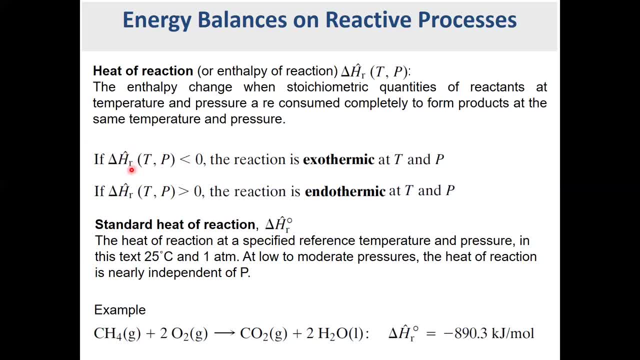 the. so in these types of process, you will the. the energy will be transferred. actually, the energy will be released from the process when the reaction proceed. this energy can may be transferred from the reactor to the heat as heat, or it may serve to raise the temperature of. 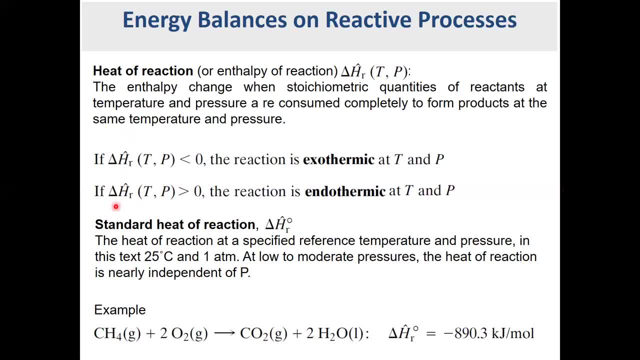 the reaction mixture. however, when there is a positive amount of heat of reaction means more energy is required to break the reactant bonds. then the energy is released when the product wants for, so leading to a net absorption of energy as the reaction proceeds. so before, actually, unless you provide this, 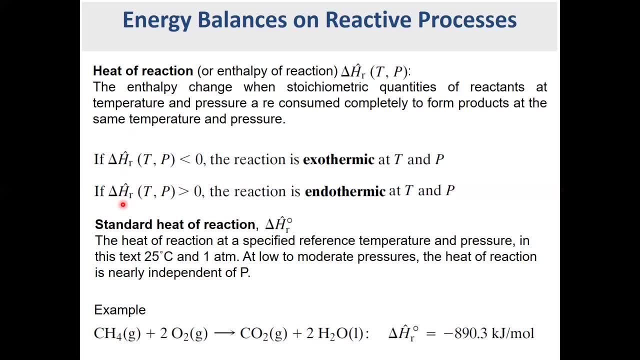 amount of the energy to the process or to the reactor. actually, the process may not proceed or the temperature will be decreased. so this is actually the heat of reaction at the temperature and pressure. however, if this temperature and pressure are specified reference temperature and pressure, they call in standard heat of reaction. so in our book at least, it is 25 degree and 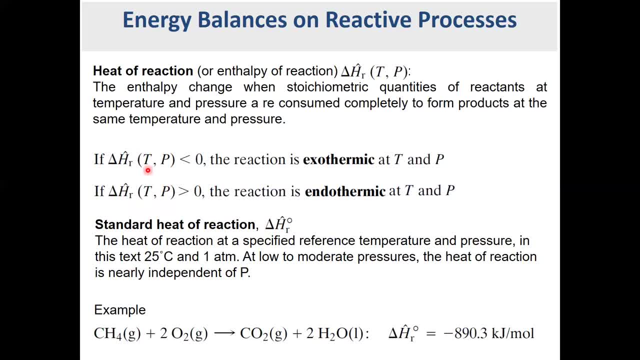 one atmosphere for this specified reference temperature and pressure. so they showing like this way: when there is a standard heat of reaction means within the when the temperature is 25 degree and pressure is considered atmospheric pressure. so so in that way you will see for by when actually one mole of methane 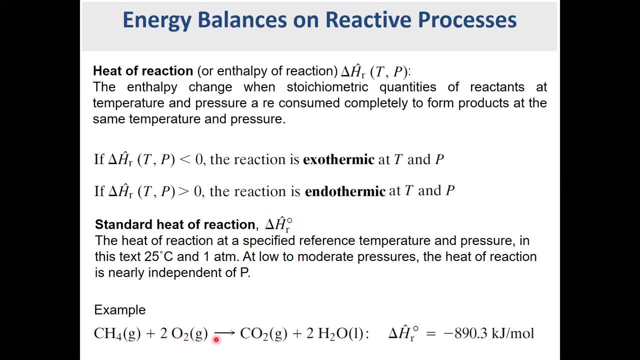 two moles of oxygen react at 25, because it is actually at standard, for at 25 degree, they will produce one mole of co2 and two moles of water at 25 degree and one atmosphere by actually this, when this reaction proceeds, this amount of 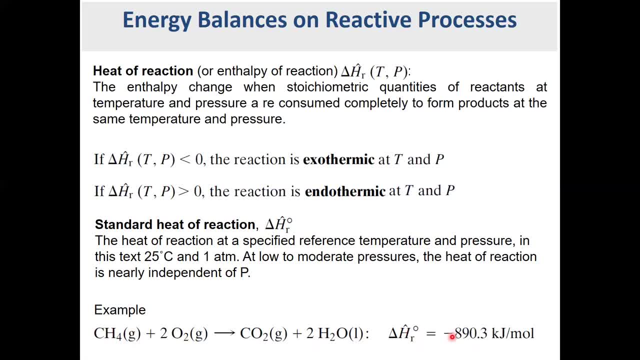 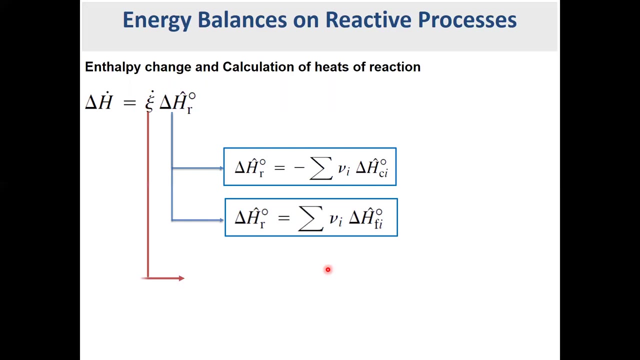 the energy will be released. since it is negative means that reaction is exothermic and this amount of the energy will be released. so actually for low pressure process you can consider heat of reaction is independent of pressure anyway. so I just want to provide for you some general equations, how to calculate different parts of how you can. you will 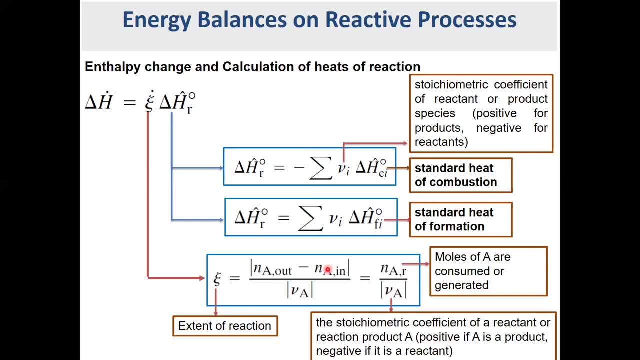 use these terms in your- we call it- study. so first of all, the changes of entropy when you have reaction will be calculated through this equation. I want to tell you: as long as this heat of reaction as 25 degree, this delta H is calculated at 25 degrees. So if you want to calculate delta H at 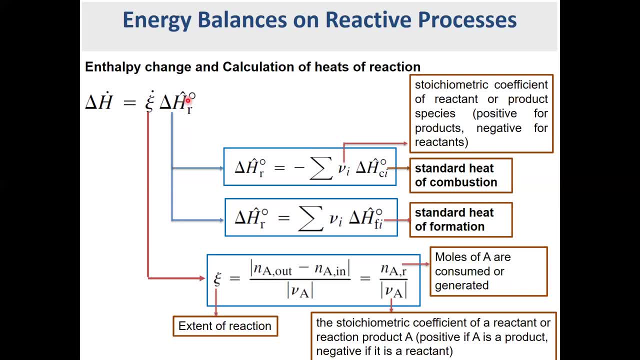 other temperatures you cannot use these reactions. So if you are using delta HR at 25 degree, this delta H can be calculated from this equation. when the process or when the calculation was asked for 25 degree or the same temperature as here, Heat of reaction, we will see. we will actually study how to calculate heat of. 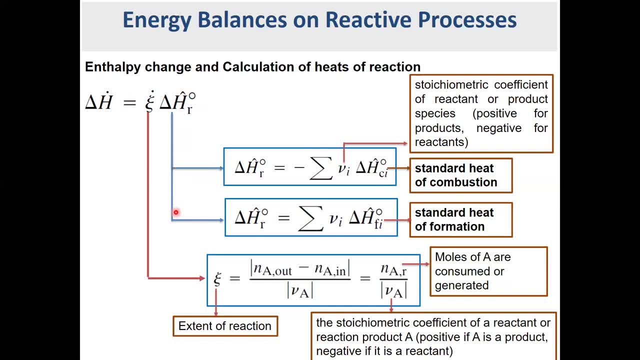 reaction so far. Maybe in some process, they give you the heat of reaction as a known data. however, if it is not known, you have to be able to calculate it through either a standard heat of combustion or a standard heat of formation. What is this value? it is stoichiometric or coefficients. 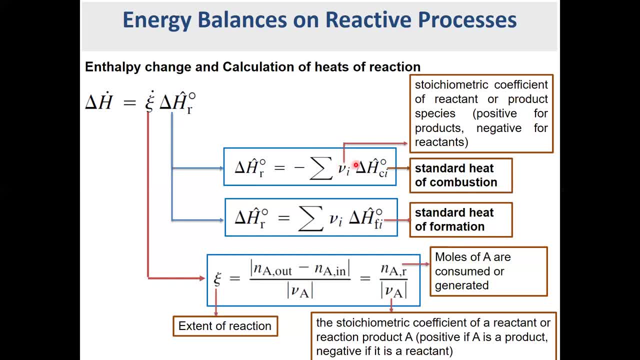 either for reactant or for product. we considered the value positive if it is a product and we consider negative values if it is a reactant. so it is a equation. if it is a equation, if you want to use, if you want to calculate a standard heat of reaction from heat of combustion, if you have the 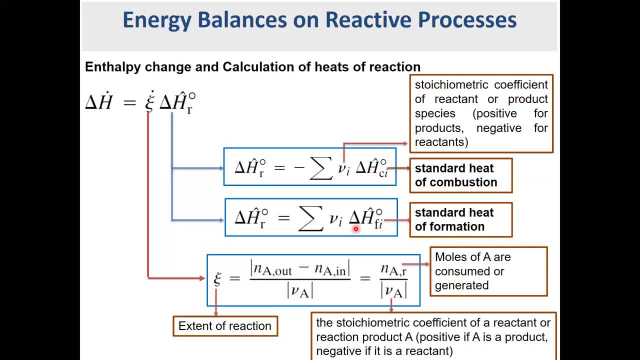 information or actually you want to use a standard heat of formation, you have to use this equation to calculate heat of reaction. so these two values. when we, when we studied chapter eight, i told you how you can find standard heat of formation and standard heat of combustion in table b1, we will. 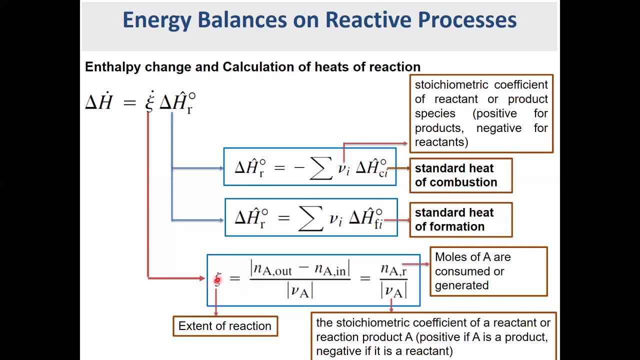 actually repeat it here. zeta, here is the extent of reaction that you studied before it show. uh, actually it is the. it show how the reactor, to what extent the reactor, proceed, so you can calculate it. if you have and the mole of any of the, you can choose any of the component in your reaction, either reactive or product. so 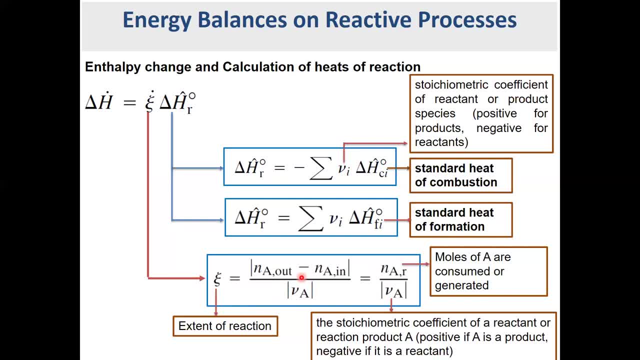 uh reactant or products. so that is known. you know how much uh the values uh at the end and at the, at the beginning and at the final. so by knowing the values, that in two values, you can calculate zeta from either any of the component of the process that you have. and again, here is actually the 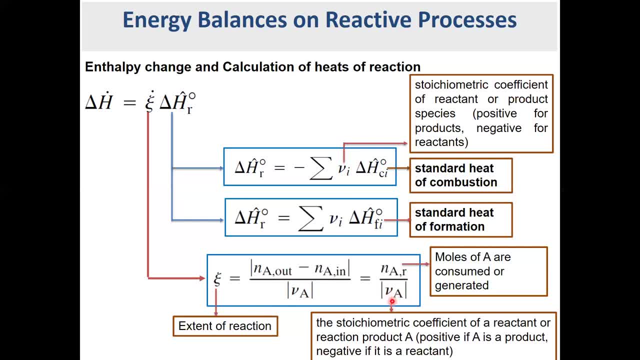 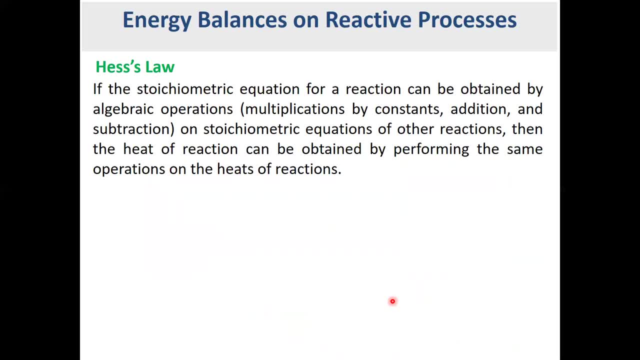 stoichiometric coefficient of a specific component that you choose, and we actually use this law in our calculation all over this in this chapter. so what Hess law tells us? we say that if the stoichiometric equation for the reaction can be obtained by algebraic operations like multiplication by addition or 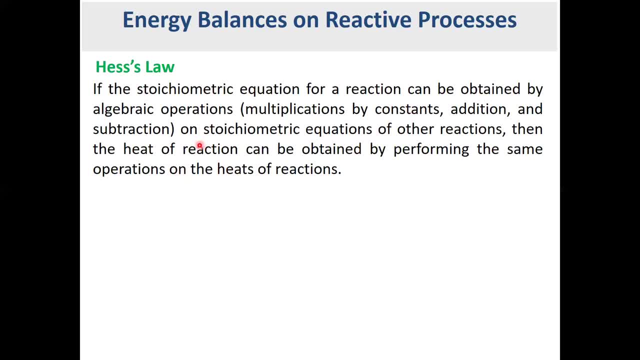 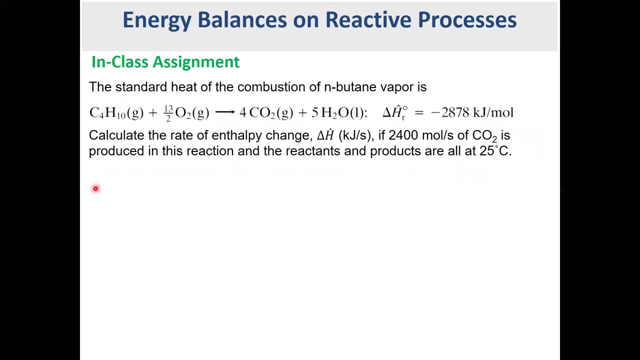 subtraction on a stoichiometric equation of other reactions, then the heat of reaction can be obtained by performing the same operations on the heat of reactions. so it's better. I show you in terms of some examples, like here we can see one, one type of actually Hess law application. 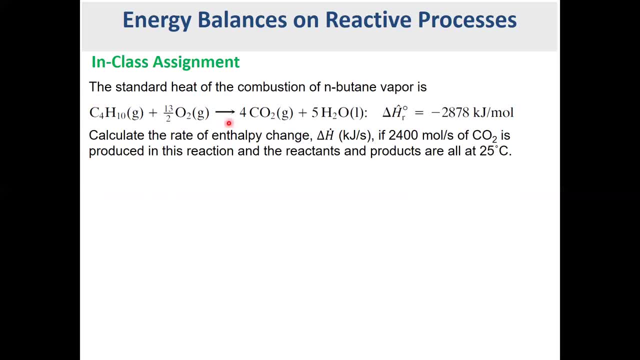 you can see one type of actually Hess law application. you can see one type of actually Hess law application. the standard heat of combustion of n-butane vapor is given to you. calculate the rate of enthalpy change if 2400 mole per second of co2 is produced in this. 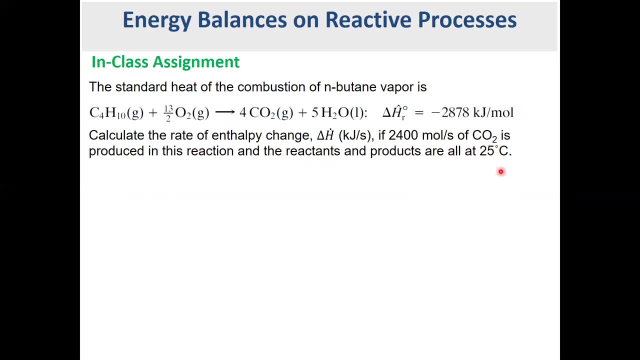 reaction and the reactants and products are all at 25 degree. so as long as it is the same temperature, we can use the equation I told you: delta H equal to zeta delta HR. so this equation is valid to use because the temperature of the process, or actually the, the temperature that we are asked to calculate the rate. 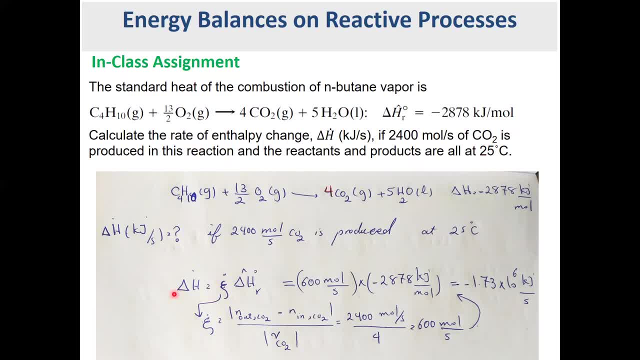 of intent into LP change is 25 degree. so we need we can use delta H equal to zeta delta HR- I mean the standard heat of reaction- and calculate the values of rate of enthalpy change. so for zeta values we can use the zeta delta HR. we can use the standard heat of reaction and calculate the values of rate of enthalpy change. so for zeta values we can use the. 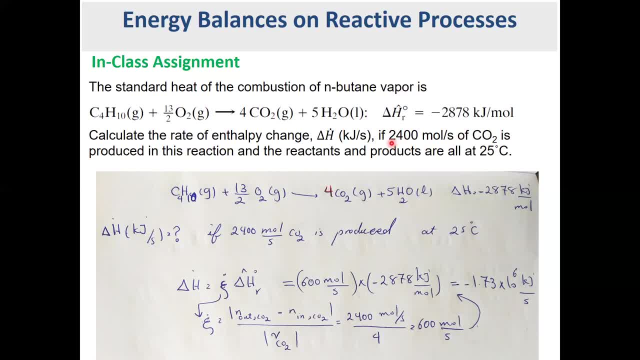 the data that is given to us. We know that 2,400 moles of CO2 is produced. There is no CO2 in the beginning, so the only values that we have in the outer stream, that is 2,400.. 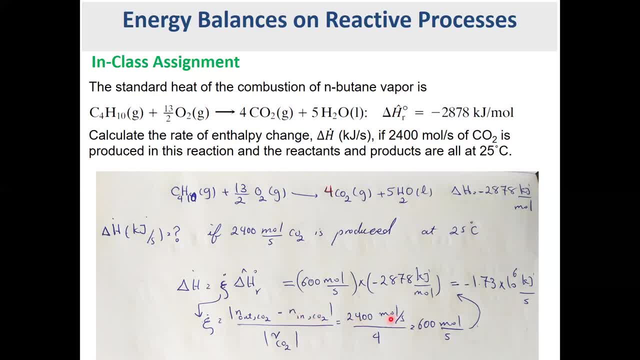 So there is no inlets CO2, so it's considered zero. We have to go to the reaction and see what is the stoichiometric coefficient of CO2, which is four, which is four. So we can actually calculate what is the extent of reaction. 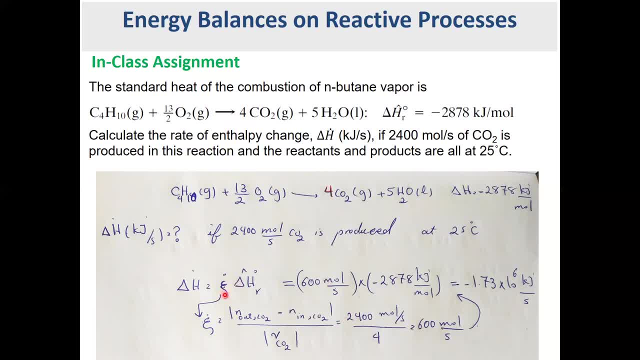 which is 600 mole per second. By knowing the extent of the reaction and the available delta H, delta HR, we can calculate rate of enthalpy change, which is this value. It was a simple process. In the other example they ask us to: 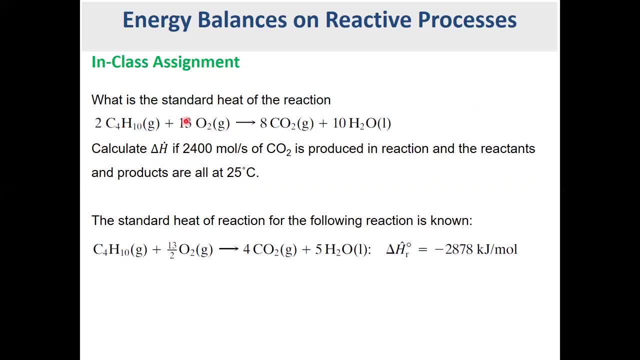 they give us the process, they give us a reaction. here They ask us to calculate the delta H rate of enthalpy change If 2,400 mole per second of CO2 is produced in reaction and the reactant and products are all at 25 degrees. 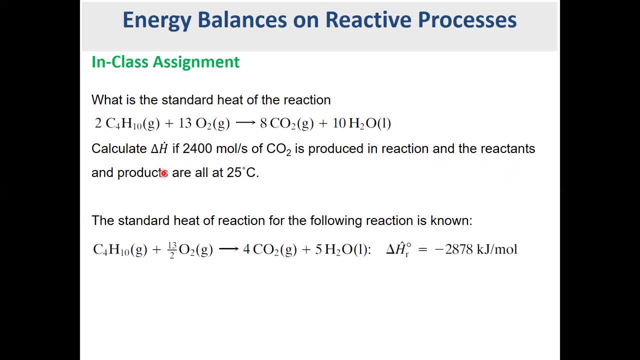 So we need actually delta HR, or standard heat of reaction, to be able to calculate the delta H at 25 degrees. What we know? we know that we need to calculate the rate of enthalpy change, So we need to calculate the rate of enthalpy change. 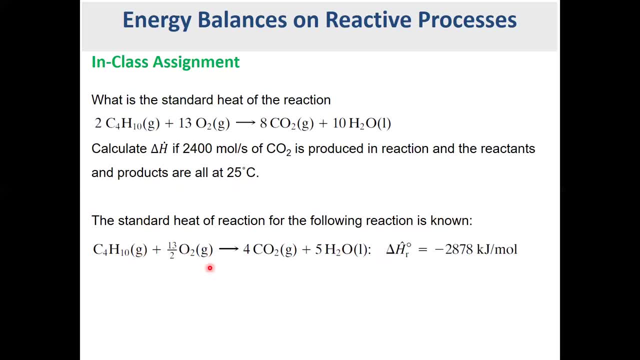 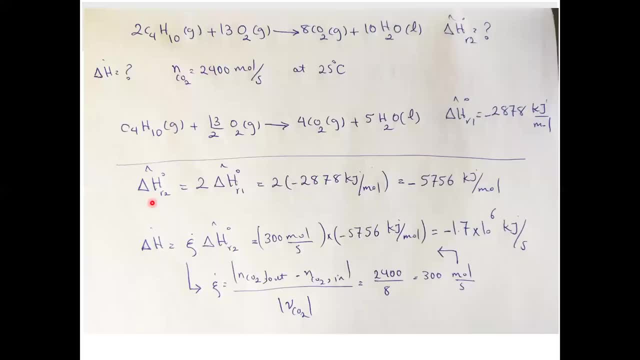 What we know. we know the standard heat of reaction of this process. So first of all we have to look how these two reactor are, we have to compare these two reactors reaction. So, as you see, we have this reaction that is asked. 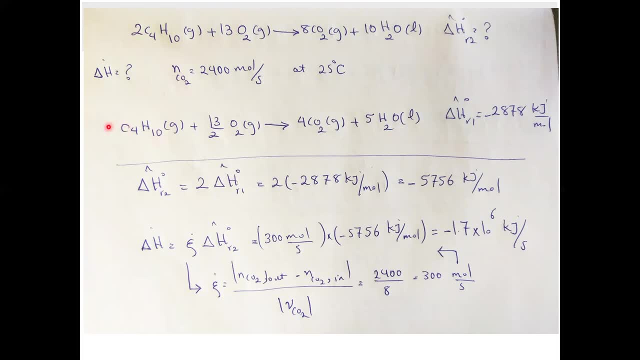 and this reaction that is given to us. What is the? if you compare these two reaction, what you will find out? This reaction is double of this reaction. I mean, if you double this document, the stoichiometric coefficients, this reaction will be happening. 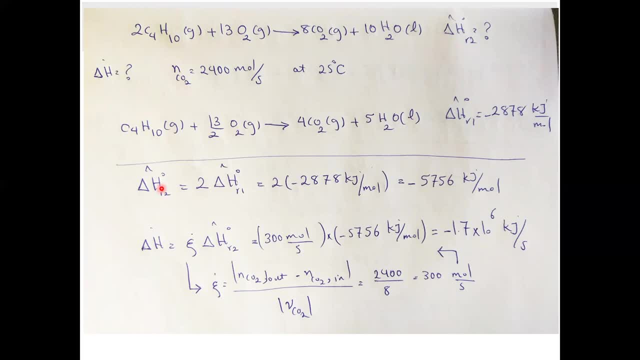 So by knowing the, even the Holtz's law mentioned, if you actually do any changes of stoichiometric values by multiplication on a constant value, you can do the same changes on the heat of reaction. So since the reaction two is multiplication of the 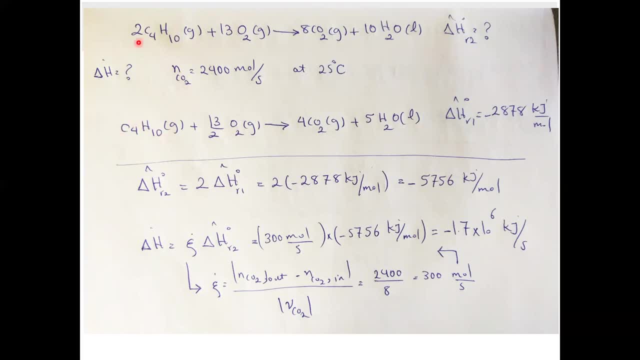 well, stoichiometric coefficient by two. we can multiply the standard heat of reaction in this equation by two. So it's just a simple thing, And I'm sure you already know about that. So we just want, we just double the heat of reaction. 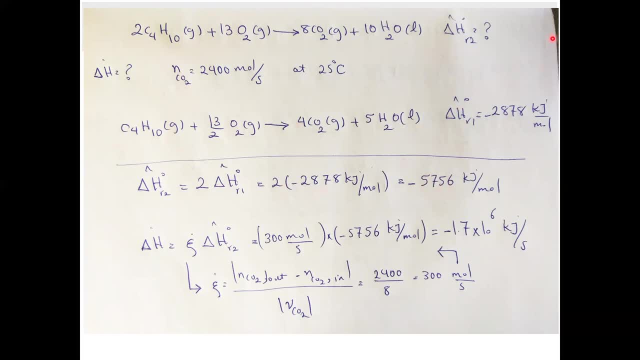 standard heat of reaction for this known reaction by two. This will be the heat of reaction of this process. So now the second terms that we need is extent of the reaction. We know 2,400 moles of of CO2.. per second of CO2 is produced. There is no CO2 in the inlet, So the 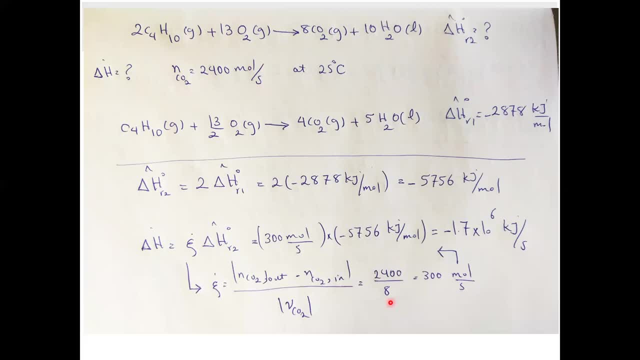 same way, we use 2400 mole per second of CO2 divided by the stoichiometric coefficient of CO2 in this reaction, which is 8. So it will be 300.. We use 300 multiplied by heat of reaction, the standard heat of reaction for reaction 2. 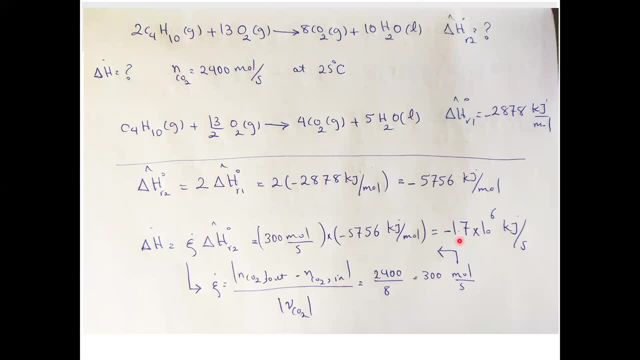 that we calculate, It is again the same value. If you compare it with the previous calculation, you will see this is the same heat of reaction, because that one is the same reaction, right? And this value is kilojoule per mole. So now 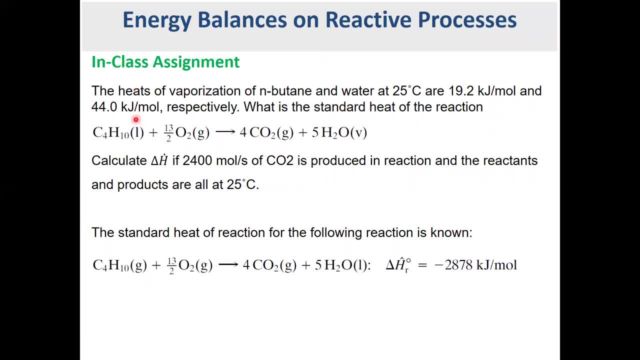 I hope that you understand so far. We have another example here. They ask us, they are giving us some information. The heat of vaporization of n-butane and water at 25 degree is given to us 19.2 and 44.. So this is the heat of vaporization of n-butane and water at 25 degree is given to us 19.2 and 44.. So this is the heat of vaporization of n-butane and water at 25 degree is given to us 19.2 and 44.. 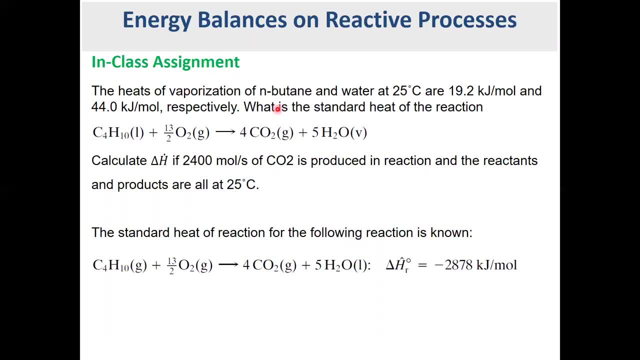 What is the standard heat of reaction? Again, we are asked for a standard heat of reaction. Calculate delta H if the same amount of the molar or actually flow rate of CO2 is produced in reaction and both reactant and product are at 25. 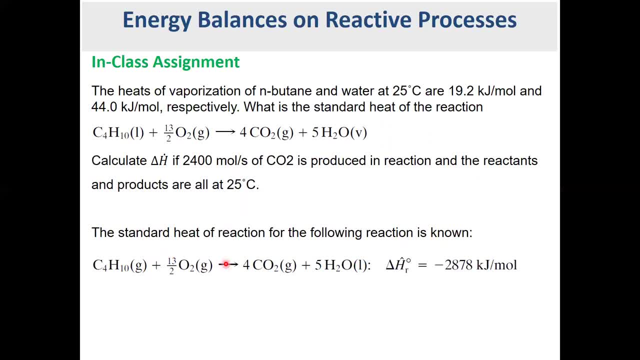 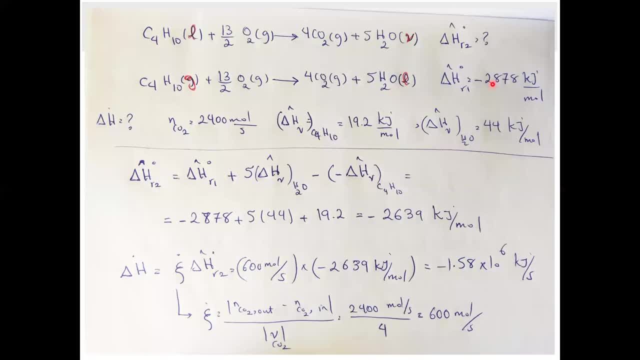 degree. Again, we are giving this the standard heat of reaction for this process. So again we have to compare these two process together, The one that is known and the one that is unknown. By comparing these two reactions we will find everything is the same. The only difference between these two reactions is the phase of H2O. 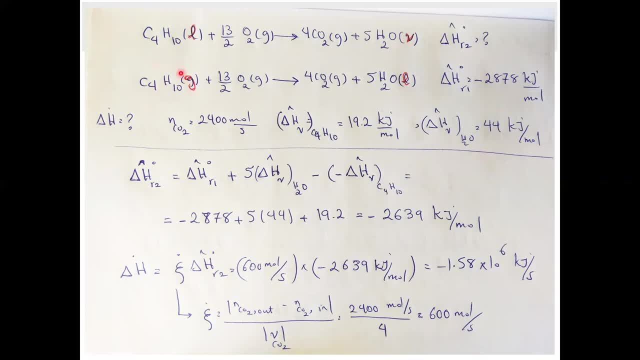 and n-butane. So what we can do, this is the information that is given to us: evaporation heat for n-butane at 25 degree and two, in this case 5 degrees at 25 degree, and for evaporation heat of water at 25 degrees. 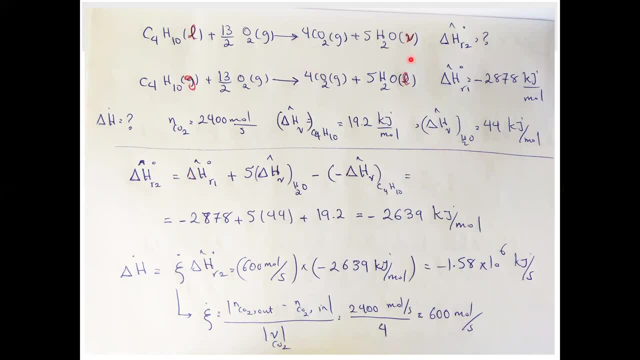 so i know these two reactions are same. the only difference here in the product you have to consider liquid version of the water. liquid form of the water has been converted to the vapor. so what you need to consider at outlet, the heat of evaporation for water. so we have to add this heat of evaporation because this 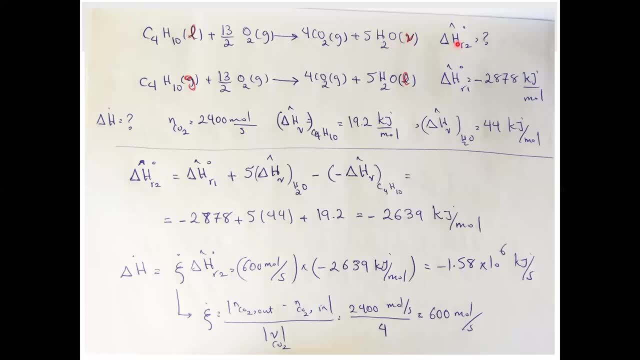 process has higher heat of reaction because of the this actually change. so i added heat of evaporation of water to this value and because it is five mole, i mean the psychometric coefficient is five. we just multiply it by five and in the reaction part you have n-butane that already converted to the liquid. 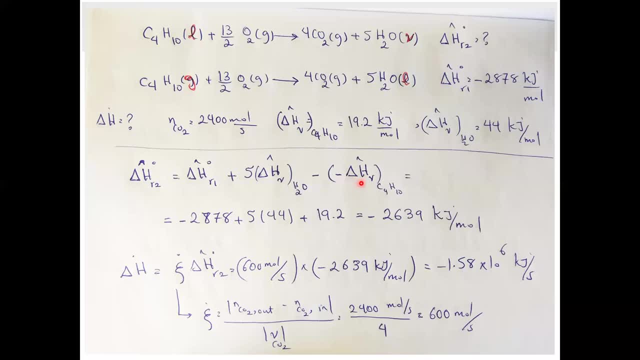 so you have to consider minus form of evaporation heat for n-butane. that is why i put minus. as i mentioned, if the value is conversion is liquid to vapor, you have to consider evaporation heat. if it is reverse form- i mean the gas to liquid- you have to consider reverse value of the. 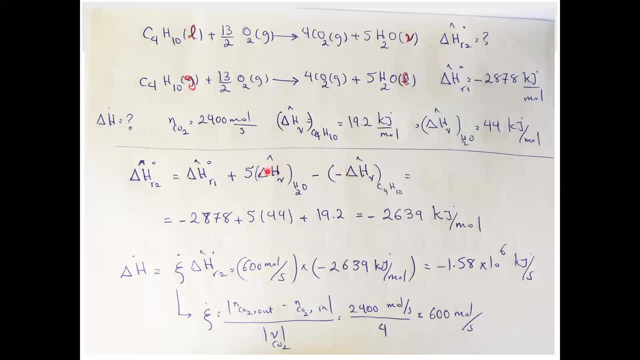 uh, evaporation heat of that component. this minus is because in delta h form we consider h of product minus h of the reactant. so minus, minus will be positive and i calculate delta h of this reaction as you have the delta h of the reaction, you just need. 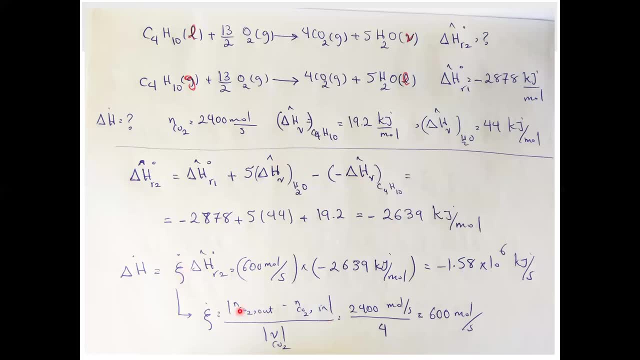 the extent of the reaction that we just calculated. it is 2400 of co2 that is produced. there is no inlet co2, so it will be an. 4 is the psychometric coefficient, and so this minus it is coefficient. We calculate this and substitute here by knowing the heat of 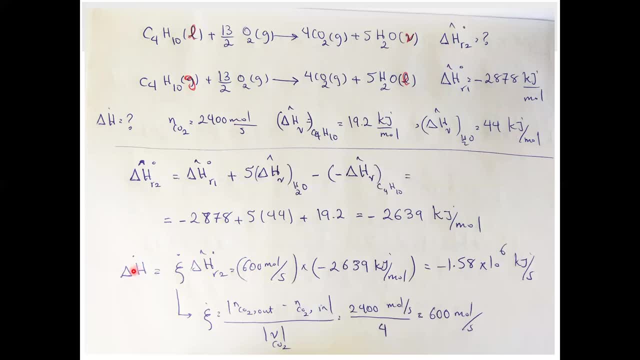 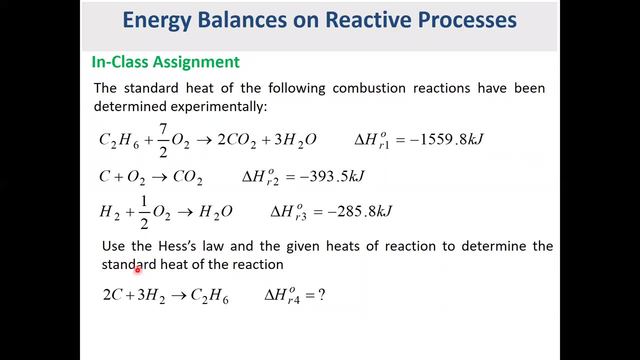 standard heat of reaction, We can calculate the rate of enthalpy change. So another example that we want to study here is a standard heat of the following combustion reactions have been determined experimentally, So we have three reactions. They ask us to use Hess law and to determine the standard heat of. 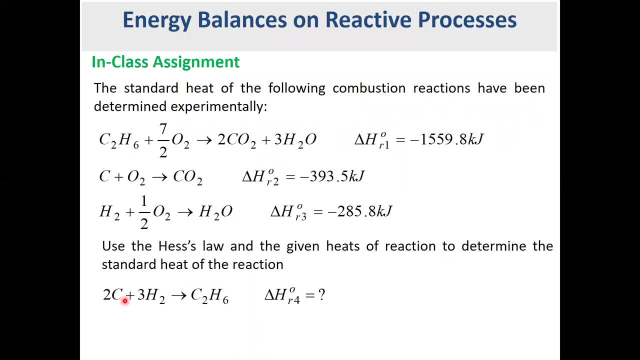 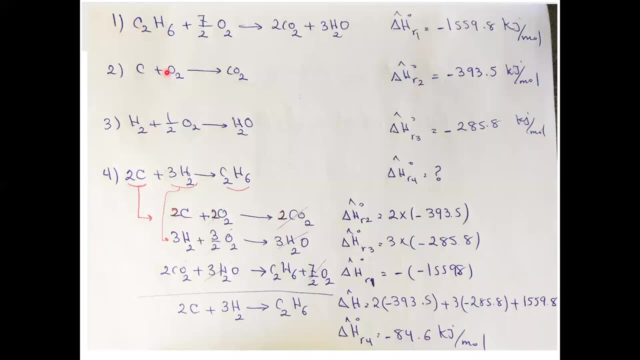 reaction for this reaction. So by using the Hess law, we have to use actually the known reaction to be able to calculate the heat of standard heat of reaction for this reaction. I just provided for you what we have in this problem. We have C, we have actually ethane here. combustion of the ethane. 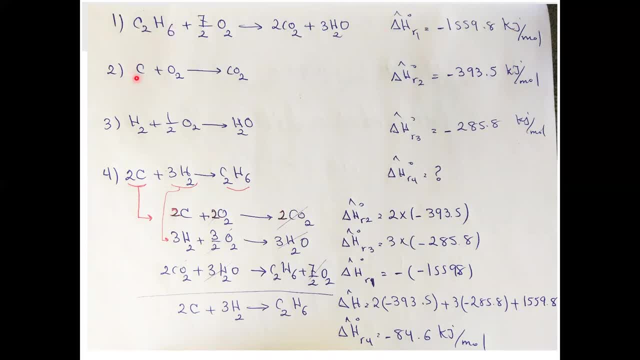 here heat of reaction is provided. We have combustion of the carbon and then the hydrogen, So we have all the heat of reaction. for this standard heat of reaction for these processes, What we are asked to calculate the heat of reaction for this process As we go through this process, we need two mole of carbon, So 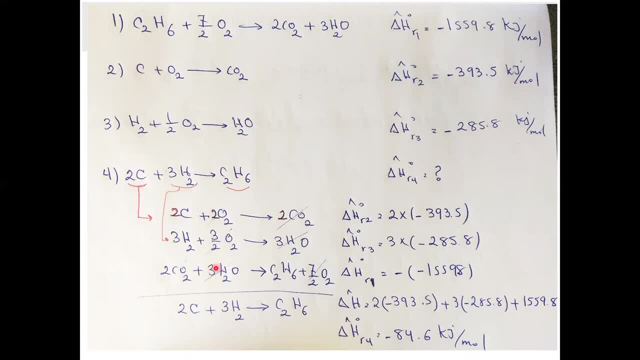 that is a reaction that we are provided. They are provided for us. So you multiply this reaction by two to be able to provide the amount we need in this reaction. As we multiply the stoichiometric coefficient of this reaction by two, we have to multiply the heat of reaction by. 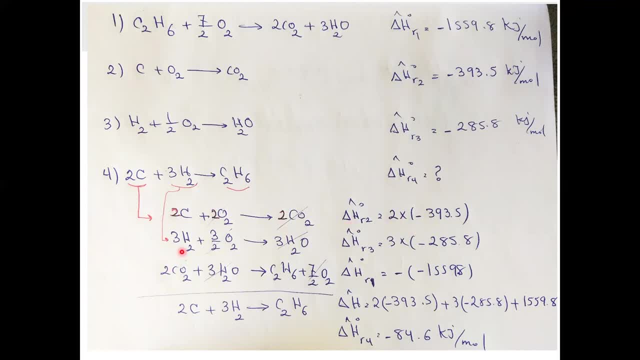 two as well. So in the second part we need three moles of hydrogen. Here we have the reaction that hydrogen is involved, which is actually one. So we multiply this reaction by three, the stoichiometric three, three, half and three. So as we multiply it by three, we have to multiply this, the standard heat. 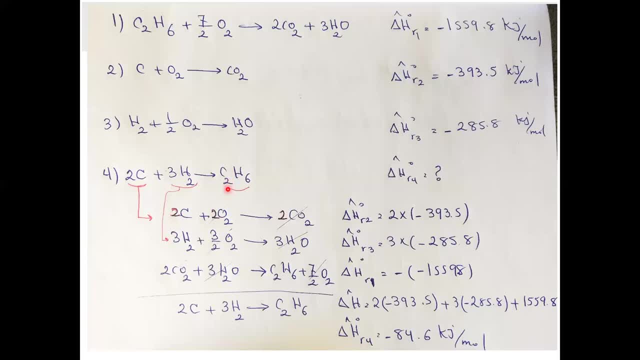 of reaction by three as well. To be able to have ethane here we have to go to the reaction involved with the ethane. So this reaction we have to just flip it, because here we have the ethane as the product, here is as a reaction. So I 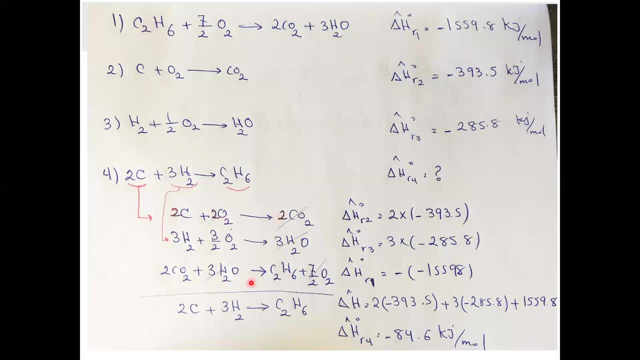 flipped this reaction. As we flip this reaction, we have to reverse the values of the heat of reaction. So we know, by this three reaction, by adding this three reaction together, we can reach to the reaction with the that is, we actually willing to it, our desired reaction, which is here. So, since the addition of this reaction, 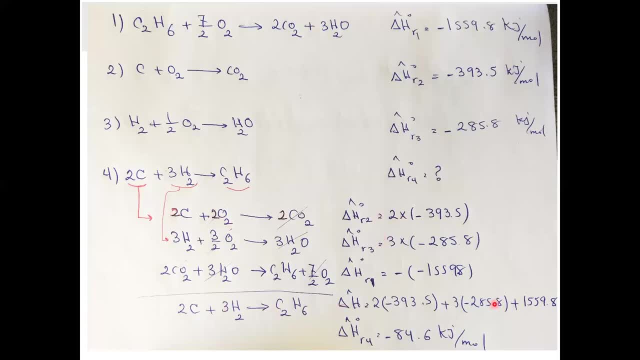 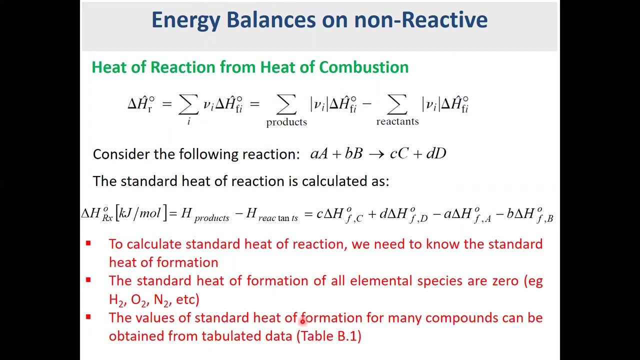 will lead to this reaction. we can add all this value now together and calculate this standard heat of reaction of this reaction by using Hess's law. So now, so far we had, we use other ways. we are giving the heat of reaction to calculate heat of reaction And 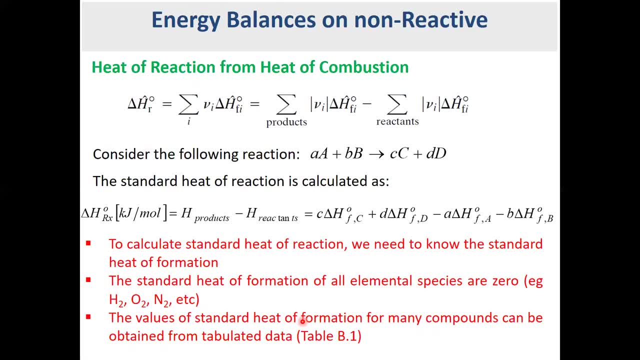 there are no other two ways we can calculate heat of reaction, which is from heat of combustion or heat of formation. So if you have a reaction like this reaction and you have heat of formation and heat of感じ, or say extra heat of of all the components of the reaction- I mean the reactant and product- you can use this. 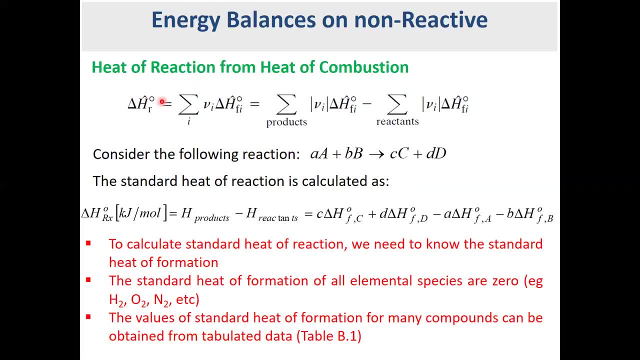 equation to calculate the standard heat of reaction. So you have to consider heat of reaction, heat of formation, standard, heat of formation of the product which is multiplied by the stoichiometric coefficient minus heat of formation of the reactants. So you just take the heat of reaction of all the components of the product. sorry, standard. 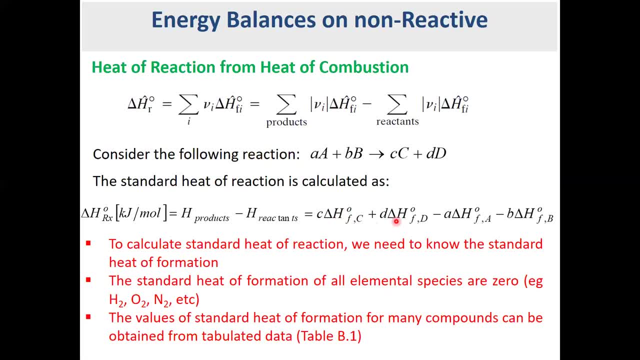 heat of formation. of this. If you remember, in the previous chapter when we studied table B1, I showed you that you have information of the reactants, You have information of heat of formation, the standard heat of formation, in table B1. So you can use those values in table B1 and consider the values you want and calculate. 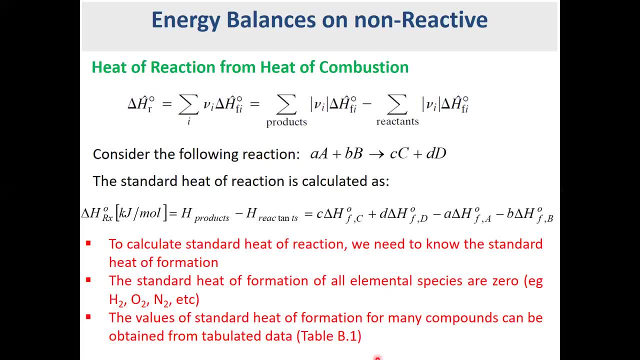 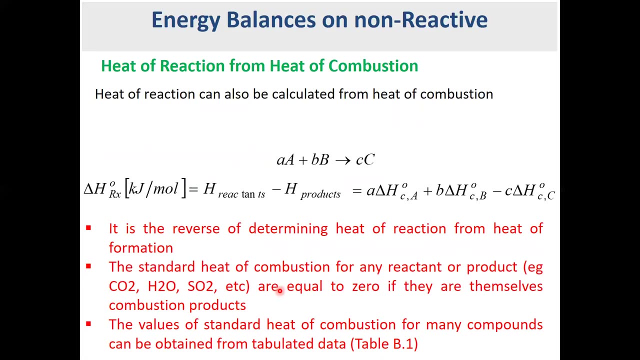 the standard heat of reaction. You have to consider the standard heat of reaction, standard heat of formation for all elemental species are zero, like H2O2N2.. Okay, More of where, if you have, if you want to calculate, both methods are available and you. 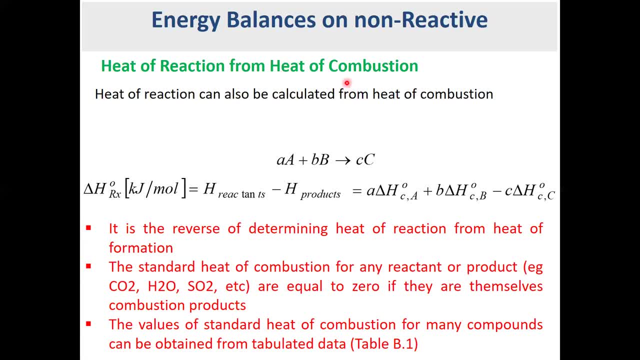 can use either of them. If you have the heat of combustion of all the components of the reaction, you have to use this equation to be able to calculate standard heat of reaction, The only difference between these two equation. here you have to know what the standard heat. 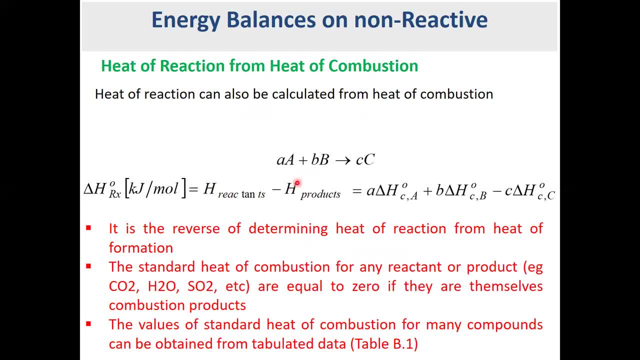 of reaction is Okay. Okay, you have to consider the Delta. H is equal to H reactants minus H products. so the same way, if you have the combustion or standard heat of combustion of all the elements, the only difference is H reactant minus H product- again this. 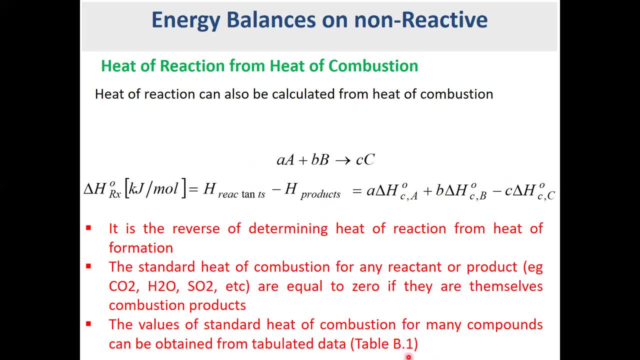 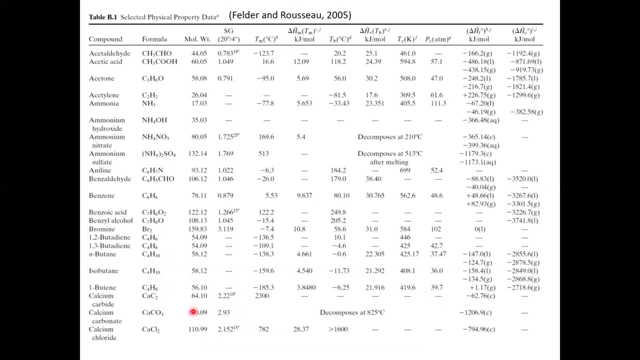 standard heat of combustion are available in table b1 in the book, in the textbook you have, and you have to consider that standard heat of combustion for any reactant or product like CO2, H2O, SO2 are equal to zero if they are combustion products. so that is the table b1 I wanted to show you in. 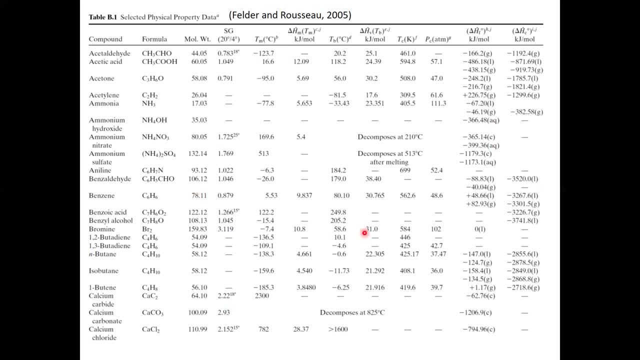 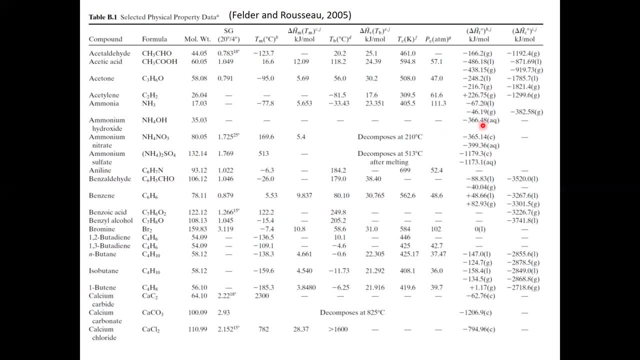 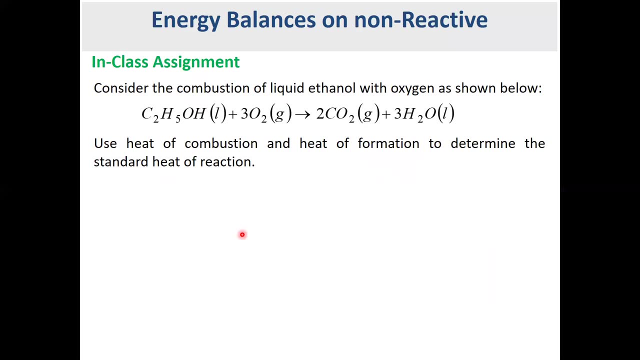 column will give you the heat of standard heat of formation and a standard heat of combustion that you can use for different components. now let's practice what we learn in some examples. so we have this reaction that we know oxygen is involved when there is a combustion reaction, so we have to use 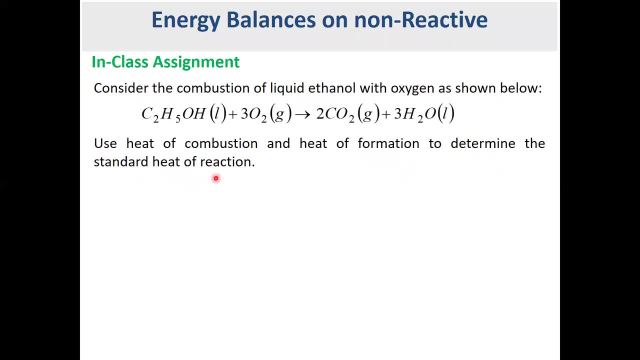 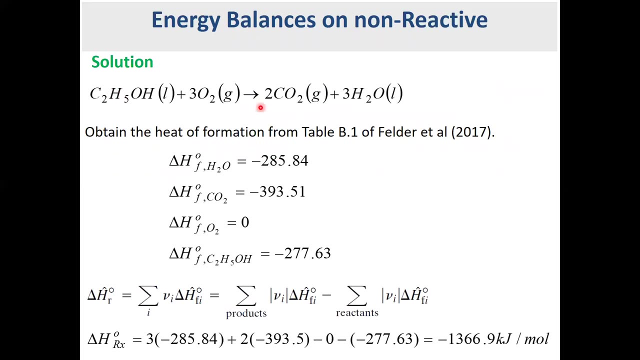 heat of combustion and heat of formation to determine the standard heat of reaction. so we want to compare both methods, if we use standard heat of formation or we use a standard heat of combustion to calculate a standard heat of reaction. so what we see here: first of all we have 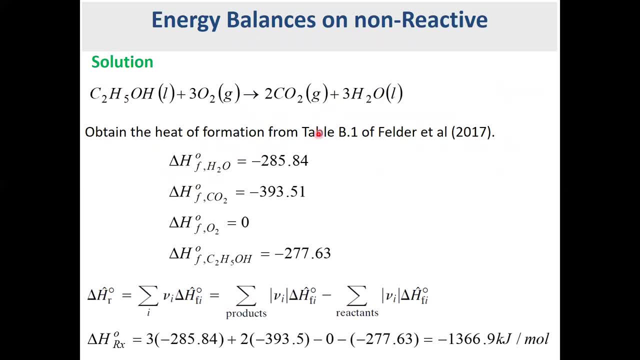 this reaction. as we know, we refer to table b1 and read all the standard heat of formation of all the component involved in our reaction. so we have one, two, three, four components. so we have it. we have all the components that are involved. we have to provide the heat of standard heat of formation of all four. 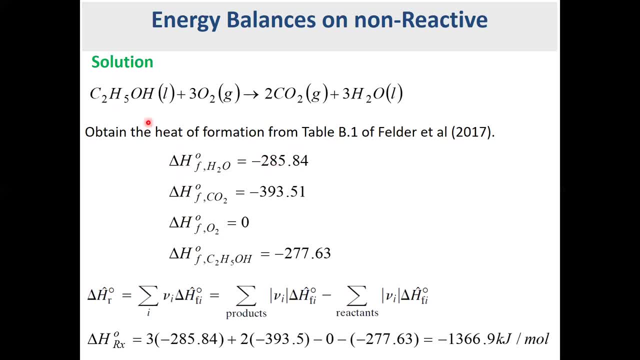 components. so we have to refer to table b1. for the first component we will find- sorry here, it is the value that you can find in table b1. for the second component is O2. we know the standard heat of formation for O2 is zero. there is. 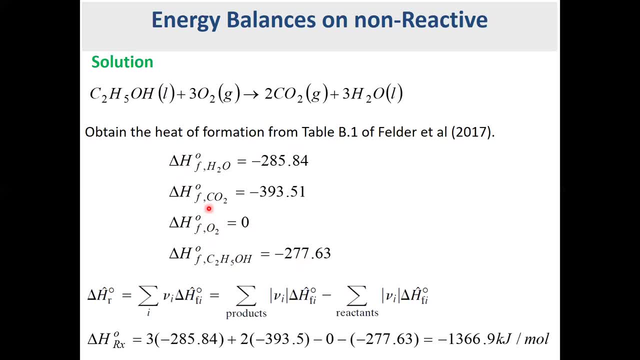 no, there is no energy for forming. there is no and there is no need for any energy to form O2 because it is available naturally as O2. so for CO2 will refer to the table and read: and the same for water. you have to consider when you are reading the data from the table. you have to consider the 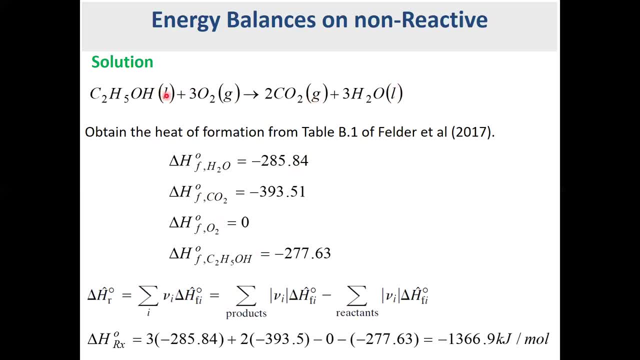 phase of each component when you are reading the data from the table. so, as we know, we just have to put it in this equation: that is a stoichiometric values multiplying by standard heat of formation for product, minus stoichiometric value multiplying by standard heat of formation for reactants. so that is why we put you see. so that is why we put you see. 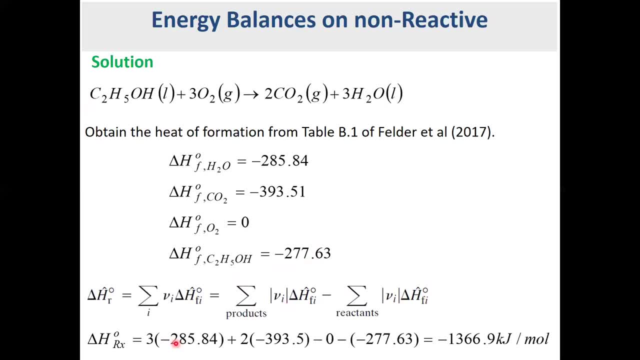 one multiplied by this value. sorry, yeah, so we have two mole of co2, so we have to, and three moles of water, so three moles of water. three is the geometric coefficient of water is 3, the values of minus 3 plus 2 multiplied by the standard heat of formation of the. 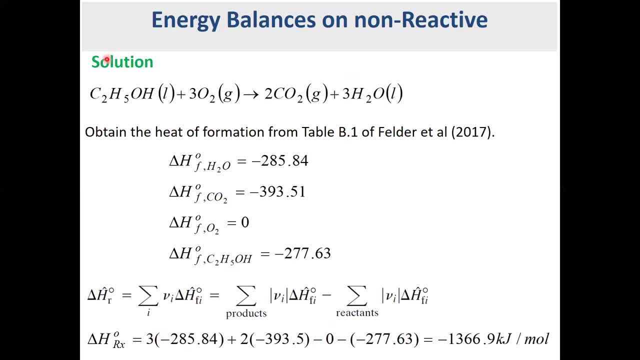 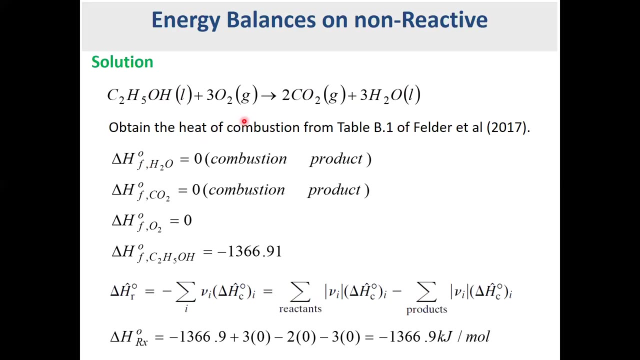 co2 minus the reactant which is here. so that is the way that we calculate the standard heat of reaction from the standard heat of formation. now, with the same reaction, we will do: we will calculate heat of reaction from heat of combustion. so here this time you go to the table and read the- sorry here, our combustion, it should. 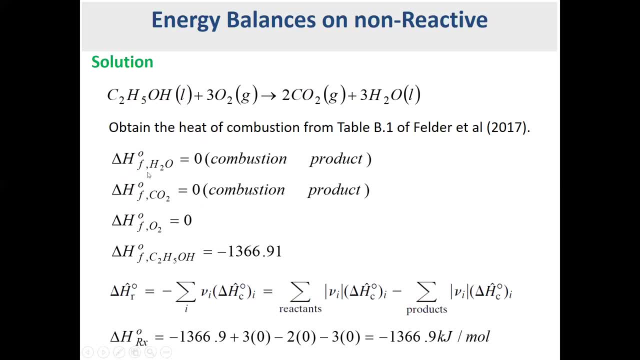 be C so you have to sorry. these values are C. it was a mistake typing. it's a typo error because this heat of combustion are all C. so for heat of combustion we know for co2 and h2o because they are when they are product combustion product you. 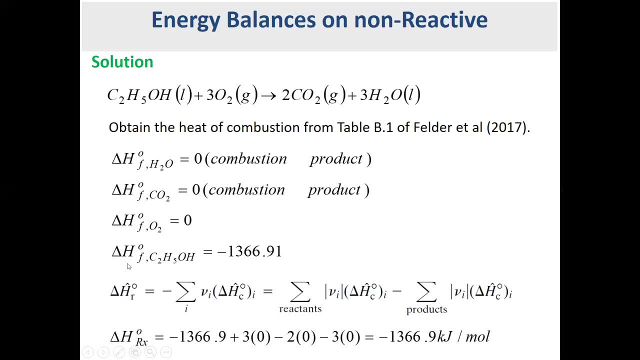 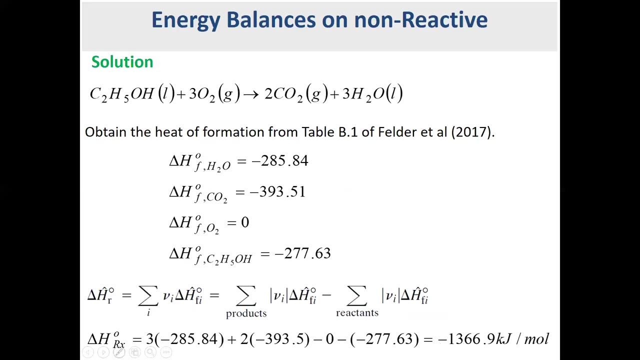 should be considered zero for all to the original heat of combustion. it is zero, and the only heat of combustion that we have here is for this component. that is minus one, three, six. so if you convert this value with the previous value, they are so close. so either you use heat of combustion, 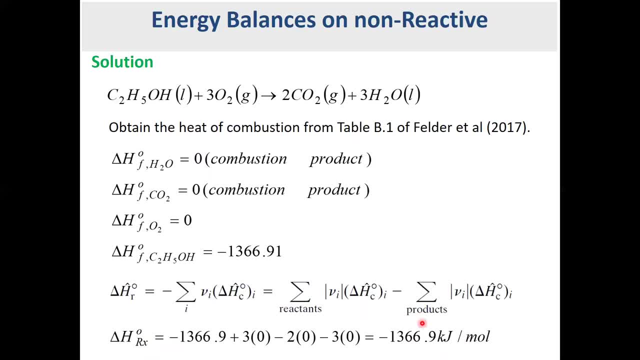 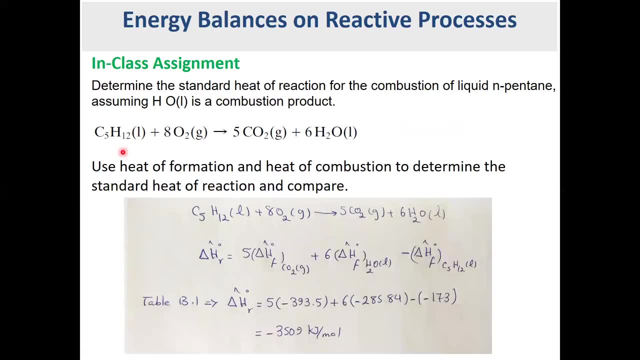 or heat of combustion method, you reach to the same value for heat of reaction. so I give you actually two assignment here, so you just practice by yourself. we have another reaction here now, so you are supposed to calculate the standard heat of reaction for this process using heat of formation and heat of combustion. 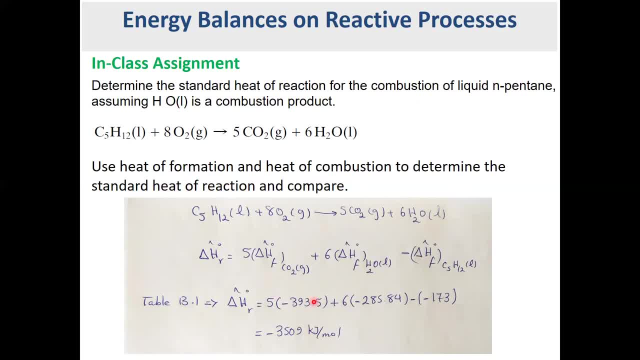 method. so here I calculate for you from heat of formation. so I give you two from heat of formation. so by knowing heat of formation we know we need heat of formation of CO2. heat of formation of water. we have to multiply by stoichiometric coefficient of these components minus heat of formation of 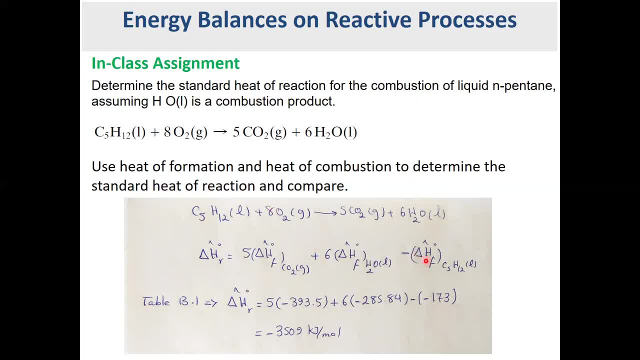 the reactants. so we need for this component, that is, n-pentane, and for O2 we know it is zero value. so by knowing the heat of formation of all these three components we can calculate heat of reaction. so now you have to go to the 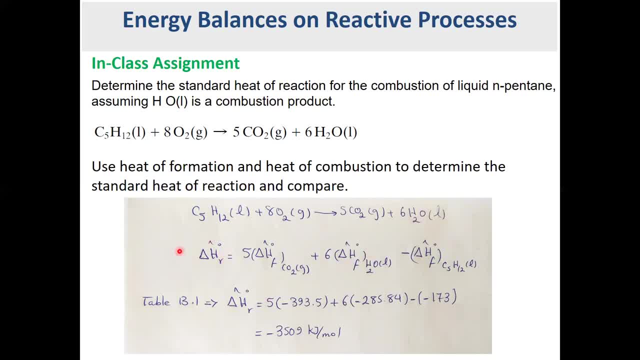 table and calculate delta H, or heat of the standard heat of reaction from the standard heat of combustion. so again, for this process, we just this one, this one, this one are considered zero as they are the product of the heat of combustion. so the only term that you have to read from the table is C5 n, actually pentane. so 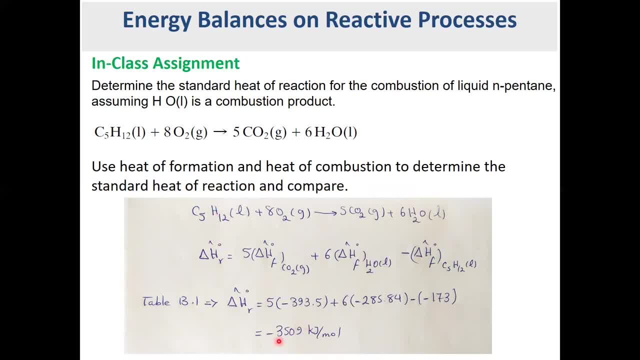 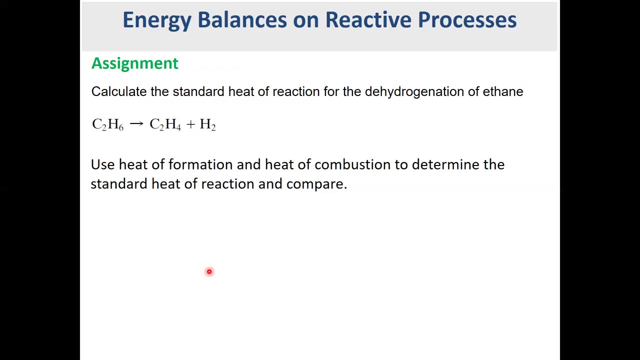 if you go to the table, you will find the value is near to this value. so please repeat to the table B1 and try to calculate heat of reaction from heat of combustion, And this is another example that you can try by yourself. So by giving you this introduction, you can actually pause this video, go and 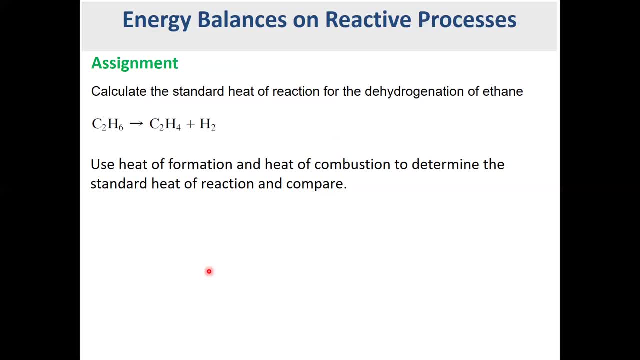 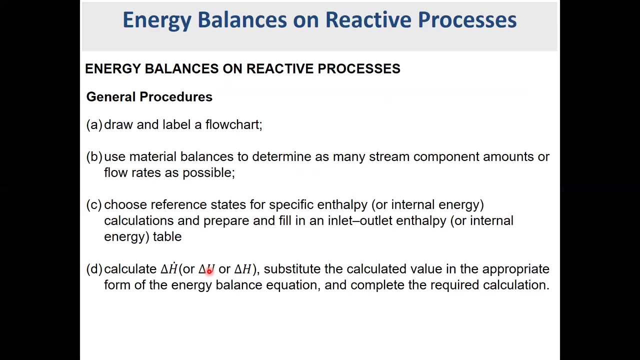 actually practice by yourself. this example I provided for you. Try to do it by yourself. just read the question and answer the question by yourself. If you have any problem, just come back to me for any more explanation or clarification. After this point now we want to go to the main focus of this. 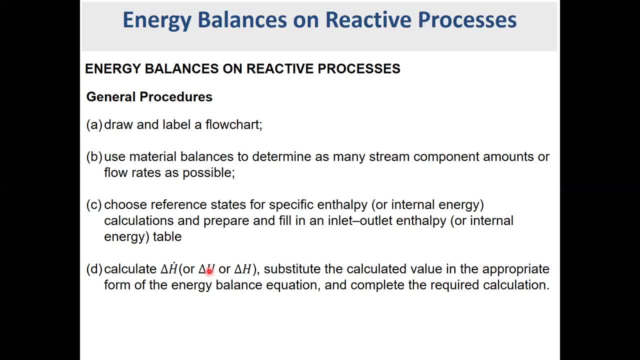 chapter, that is, energy balance on reactive process, When there is a reaction involved in the process. how you have to do energy balance. First of all, a general procedure that you have to do. As always, you have to draw and label the. 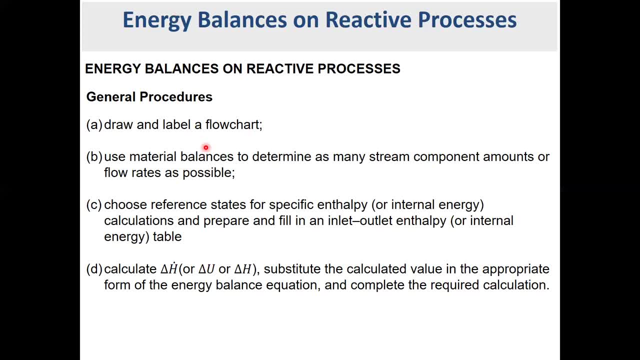 follow chart. You have to draw the follow chart of the process and actually draw it and actually put all the information that you have. So, as usual, we have to do a material balance, as we have, As we have the values of a material balance and as we can calculate. we have to do all of them and 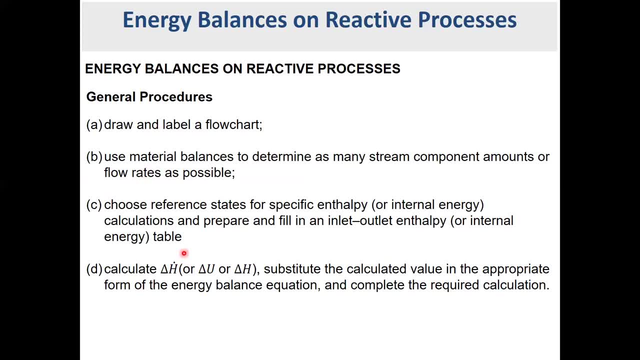 provide this value in the follow chart that we provided. We should actually provide the reference state for a specific entropy or internal energy. This reference state- as I told you in chapter 8, is a compensatory part of the process, because you need reference state to calculate the. 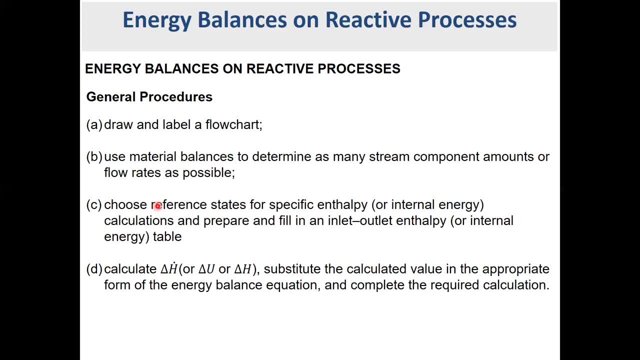 specific entropy or internal energy. After you provided this reference table, it is recommended that you provide the inlet-outlet-entropy table, as we provided and actually we practice now. And finally, as you have all the components that you provided, this inlet-outlet-entropy table, you can. 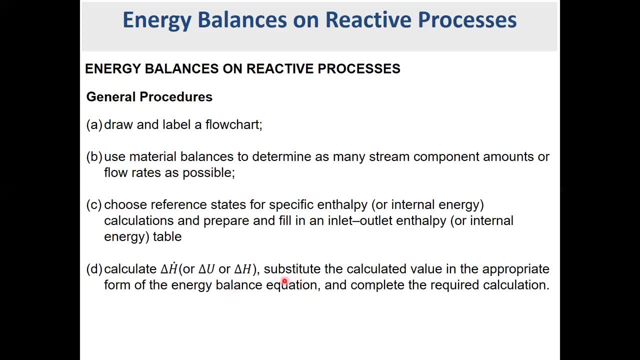 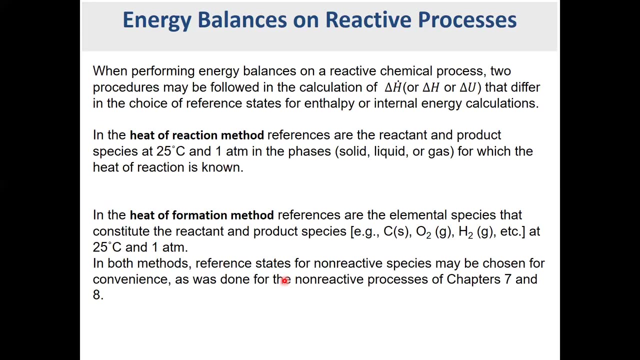 easily calculate delta H or delta U depends and just put it in the final equation of energy balance and calculate the term that you need if it is heat transfer or other terms that you may need When you are doing the energy balance on a. 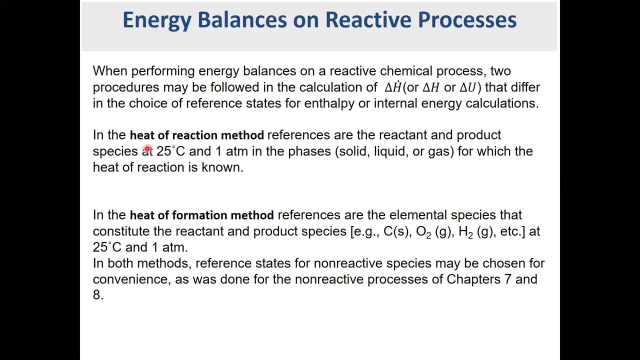 reactive process. you can either use- you can actually you have two methods for your calculation. You can use heat of reaction method or heat of formation method. We will practice both methods on one actually process. The difference between these two methods is the reference point. 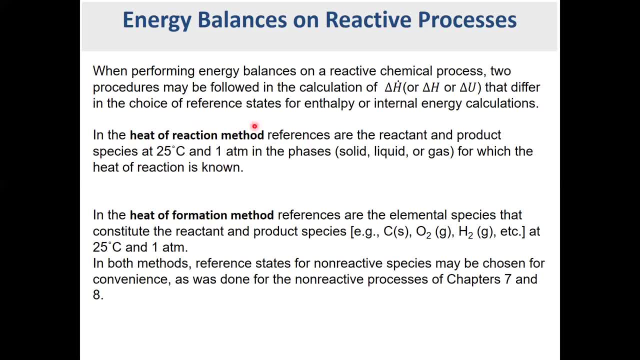 When you're using heat of reaction method, your reference point will be all reactant and production at 25 degrees on one atmosphere in the phase that is existing in theوي temperature and pressure For reactant and product. you have to use this reference. 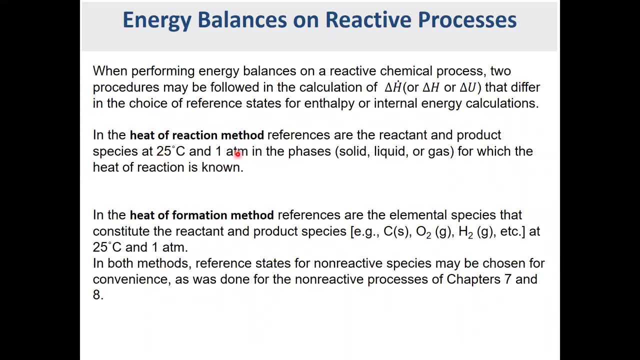 point for nonreactive components, you can use any reference point you want. depends on you. even you can use this reference point, You will practice, While if you are using heat of formation method, you have to consider elemental species that constitute the reactant and product species at 25 degree and 1 atmosphere as 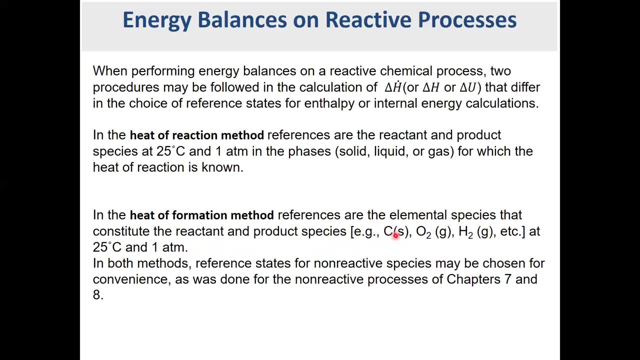 your reference point. What does that mean? Carbon as solid oxygen, actually as a gas form, hydrogen as a gas form? They are the elemental species that are available in this condition at 25 degree and 1 atmosphere. So most method are applicable. 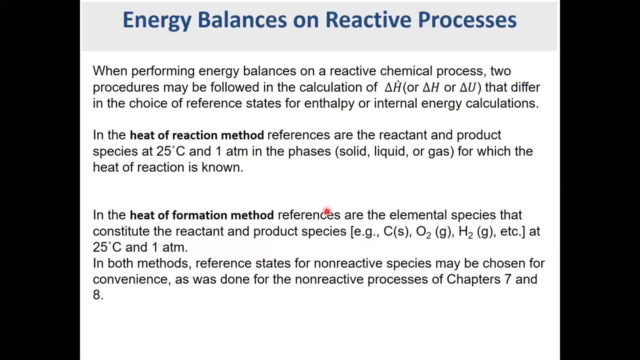 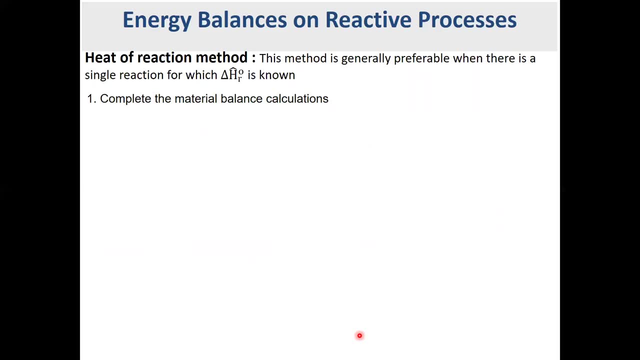 Sometimes depends on the situation. One of them is easier to apply and other one may be a bit more challenging, but you can use either two methods for your calculation of the energy balance and reactive processes. So let's start to understand, if you want to use heat of reaction method, what the steps we have. 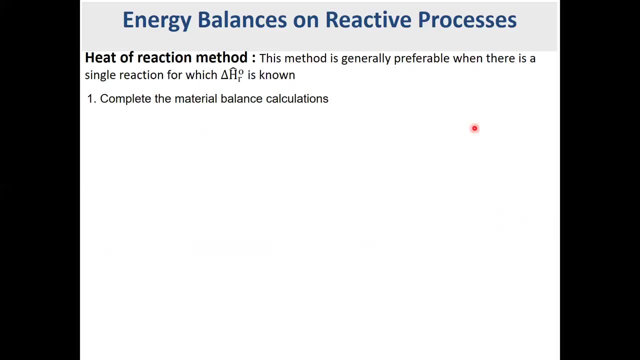 to follow. so heat of reaction method. before we study about the steps, let's see how, in what condition is better, we use a heat of reaction method. usually it is preferable for you to use this method when there is just one reaction involved in your in the process and a standard heat of reaction is known. or you can 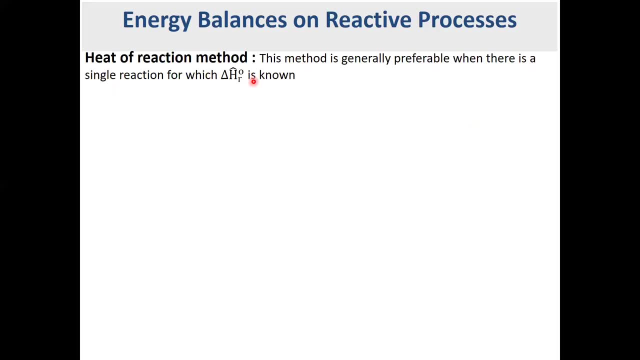 actually easily calculate it, as we just show you different methods. so it is preferable, right? so you can actually. that makes the calculation easier for you when there is just only one reaction involved and a standard heat of reaction is known. or you can easily calculate it somehow. it is not easy to calculate. 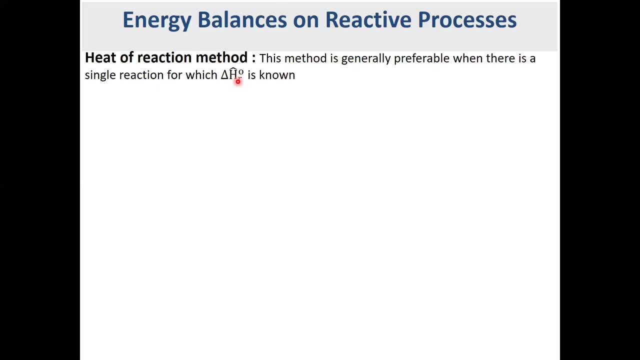 because the temperature of the inlet and outlet is not 25 degree. we know we can calculate the standard heat of reaction only for 25 degree. for other temperature is not easy to calculate. so if a standard heat of reaction is known and if you just have one reaction involving process, it is better to select heat of reaction method. 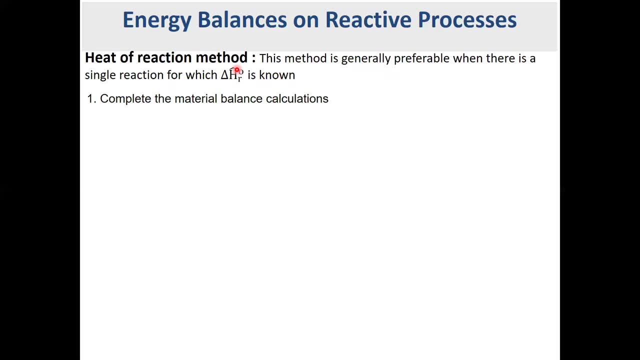 so what are the steps you have to follow? as we always mention, you have to do a good material balance on the system for each reaction on a particular set of reasons- n whatsoever you have. You just provide the material balance with the known data. or, if you can calculate, just add it For sure, you have to draw the flowchart. 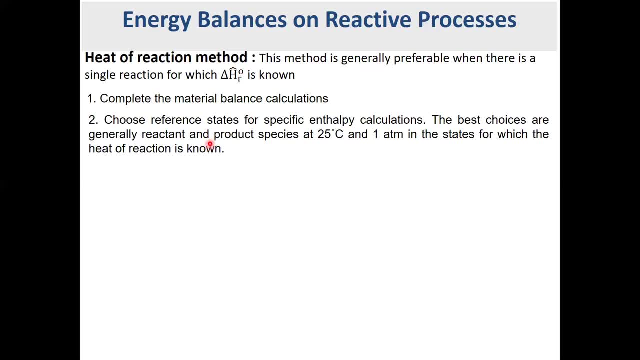 before this. Then you have to choose your reference state. A reference state for heat of reaction method, as I mentioned, is clear. You have to consider all the reactants and products at 25 dp and 1 atm In this state. they are available in this condition. So we know this temperature and pressure. or 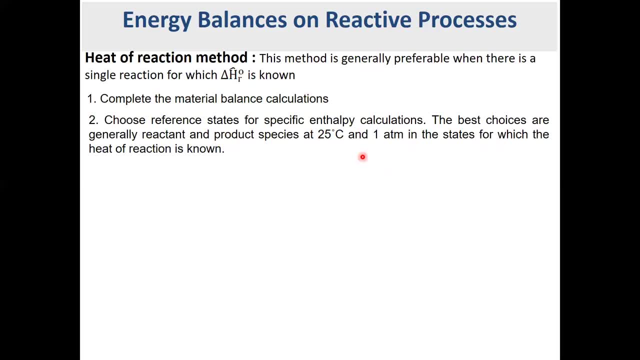 the same temperature and pressure of the heat of reaction. That is why we use this point as the reference point. As you provided these two conditions or you actually follow these two steps, you have to calculate extent of extent of temperature. So, as you calculate this and follow this step, 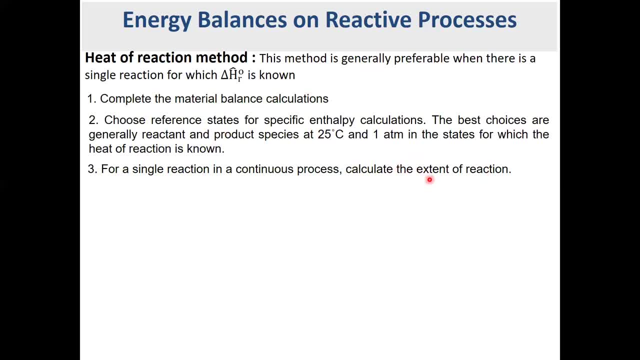 extent of reaction. Extent of reaction is easy to calculate. I'll show you. You can select any of the reactant or products that it is available in. You have all the information of the inlet and outlet flow rate, molar flow rate or flow rate, and. 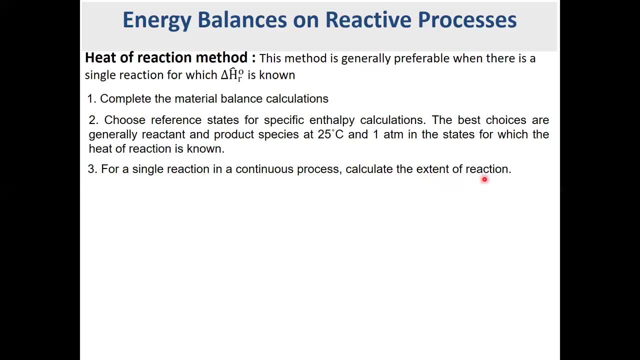 you can easily calculate extent of reaction. Then provide the inlet outlet enthalpy table and put all the values you have for material balance, for energy balance, all the value you have put it in that table. And if you have any of the component at 25 and 1 atmosphere you can select the enthalpy of that component. 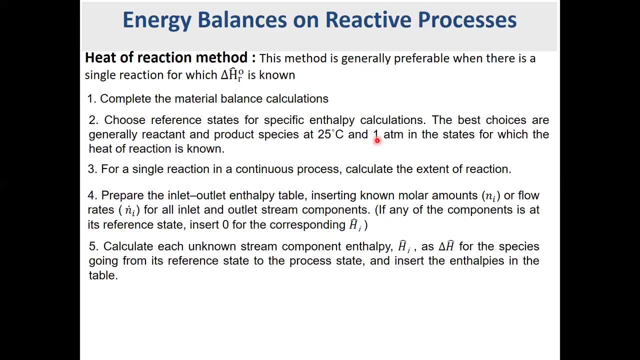 0 because it is the reference point. So after you provide this table, you know which component actually the enthalpy specifically. the energy balance is the reference point. So after you provide this table, you know which component actually the enthalpy specifically. 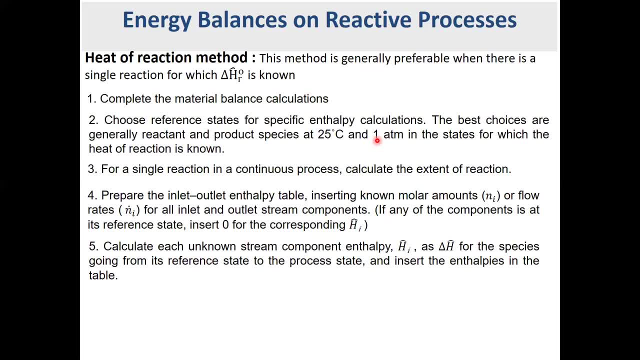 the energy balance is the reference point. So after you provide this table, you know which component actually the enthalpy, specifically internal energy, depends on the process. It's unknown and how you can calculate it based on the changes from the reference state and the information. 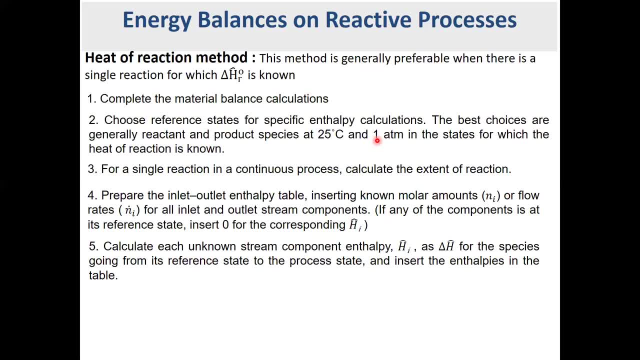 that you have, or tables and the process you have to employ. After you have all the information, it is easy to follow up. You can use: if you have single reaction, you can use this process. this actually equation. if you have multiple reaction, you can use. this actually equation. So extent of 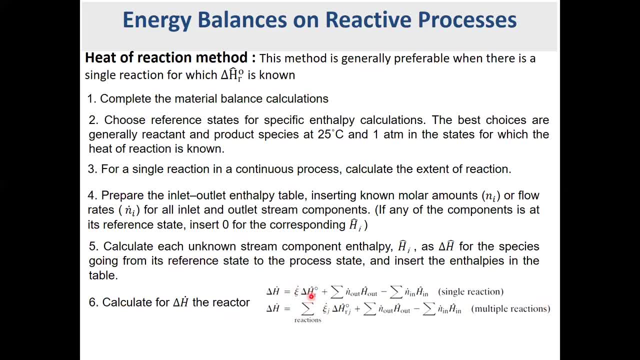 reaction, the standard heat of reaction and old. actually, This is a part we did in chapter 7 when there was no reaction. So the only difference that you have here: when you have reaction you have to add it to the delta H equation. So this is actually you can get from the table that you provided and 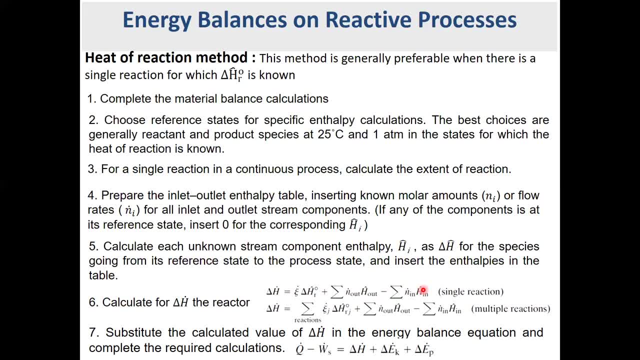 already calculated the equation. So this is actually you can get from the table that you provided and already calculated all the H involved in the system. Finally, you can just put the values of the delta H you have in this energy balance equation. that is for open system, for sure you have for closed system you. 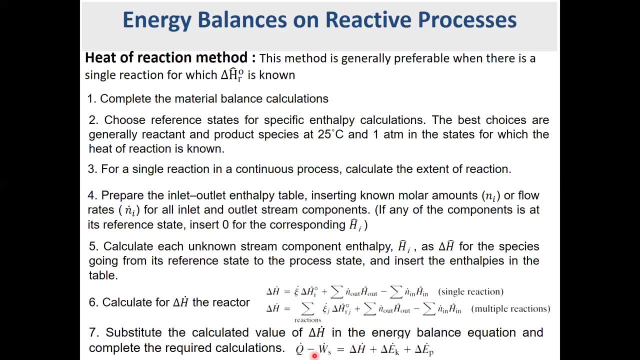 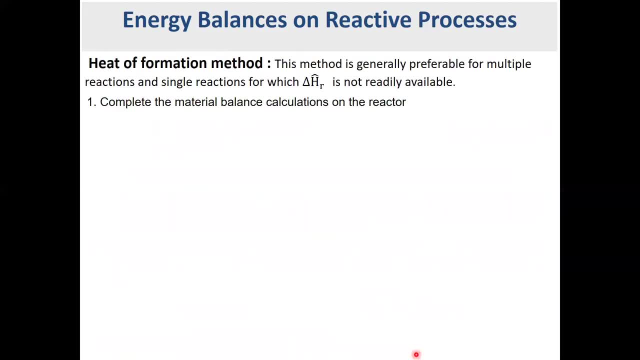 know. So you can just substitute the values that you have and if you want to calculate heat transfer or any other component that you want, you can easily calculate For heat of action formation method, this process, we use actually this method when we have multiple reactions or when you have a 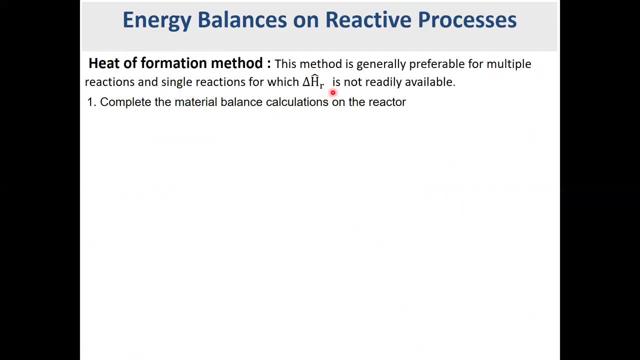 single reaction, but the standard heat of reaction is not known, it's not available. so you can use this method in that process. you will see you by actually going through the example. you will find out why it's easier. same way you have to start. you draw the follow chart, complete the material balance and calculate all. 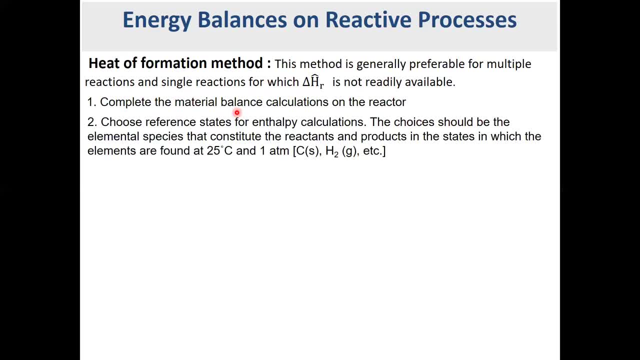 the material balance that you can provide in the follow chart, and then your reference state for heat of formation method is clear. you have to use elemental species that constitute the reactant and product in this state, in which elements are found at 25 Celsius and one atmosphere, which is for 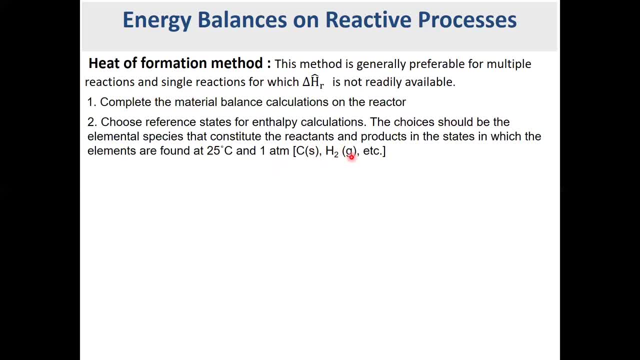 carbon, its solid form for hydrogen gas form and actually for other o2 in gas form, hydrogen in gas form. these are the elements that found a 25 degree and one atmosphere, and you have to form those components involved in the reaction from these elements. so then you have to. 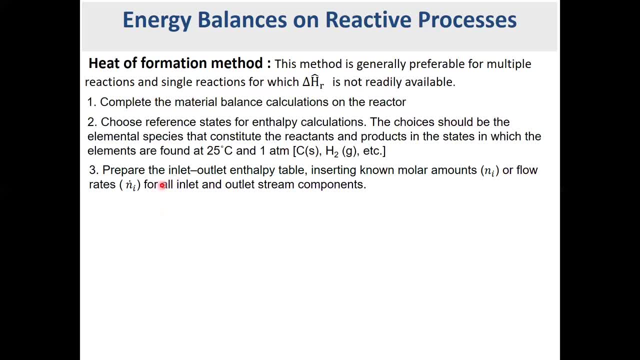 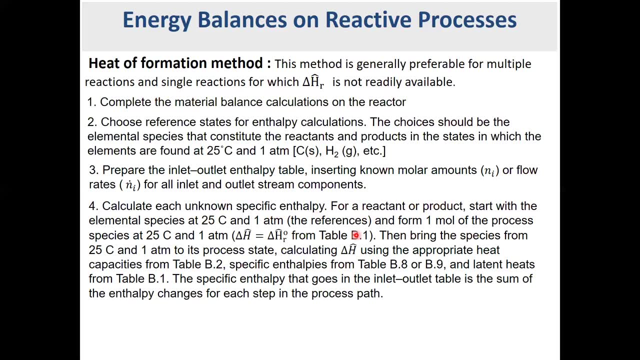 provide the inlet-outlet enthalpy table and provide all the information you have and then calculate. as we mentioned, you have to calculate a specific enthalpy here. we are talking about open system, just for example. so you have to calculate all the specific enthalpy for the unknown problem. so I think it's. 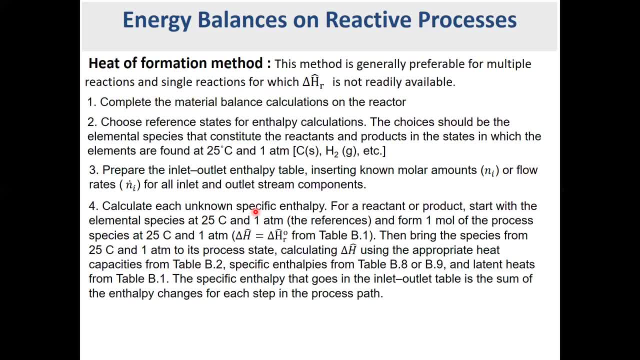 better. I show you in the example how you can provide this one. but as you learn so far, heat of formation at 25 degree and one atmosphere is available in the table. so means heat of formation. this heat of formation is when the specified elements are actually reacting together and form that specific component. so in table B1. 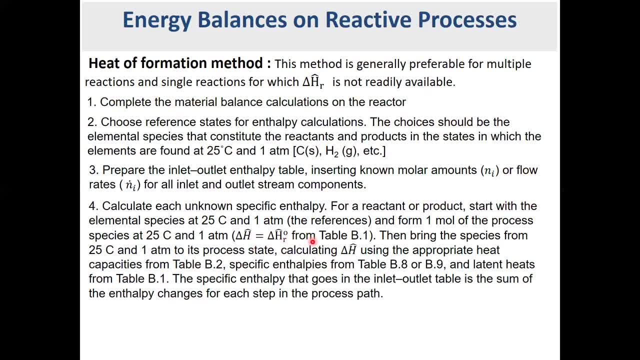 you can read the heat of formation: standard heat of formation at 25 degree and one atmosphere. however, if the component is not formed, then the heat of formation is not formed, then the heat of formation is not formed. and the heat of formation is not formed, then the heat of formation is not formed. 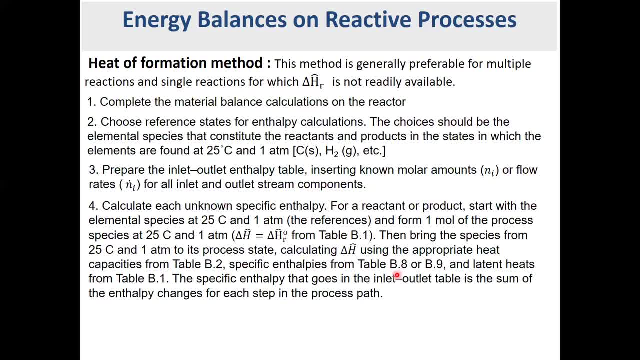 in your reaction have other temperature and pressure, you have to do further calculation to calculate those values. so you may use table B2, you may use the food be 8 or be 9. in this we will explain how at the end you just can put in the simple equation that have so far and calculate rate of. 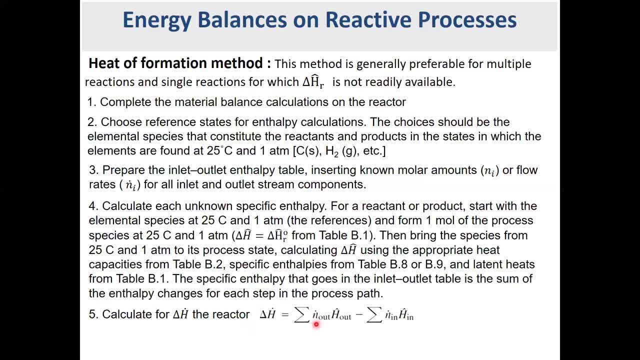 internet change. so we don't need. if you, if you focus here, you would see we don't need the standard heat of reaction or heat of reaction in our calculation for heat of formation method. That is why we use this method, because it's not our concerned value. And at the end, as you, 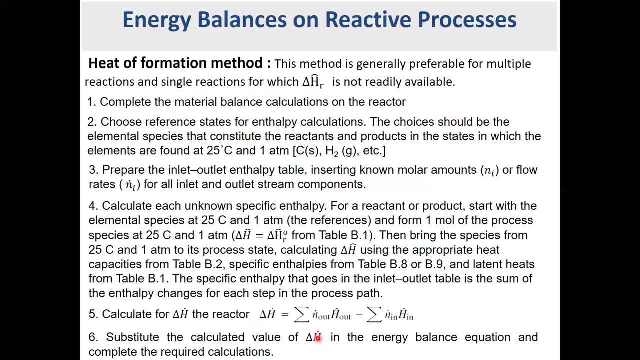 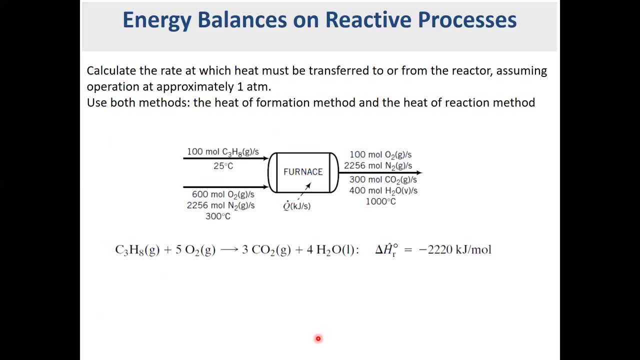 have the values of delta H you can put in the energy balance form and calculate what it is. If heat transfer or whatsoever you need, you can calculate. So now it's better to go to one example and see how we can do this energy balance on the. 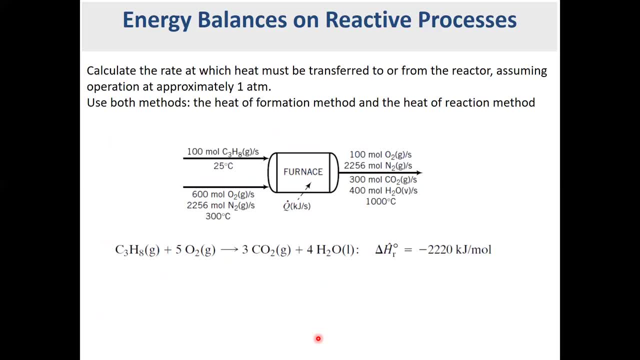 reactive process by Bohr's method. So you have, we have a reactor here in form of a fairness, We have some inlet streams, some outlet streams. So we want to see and we want to calculate the rate at which heat must be transferred to or 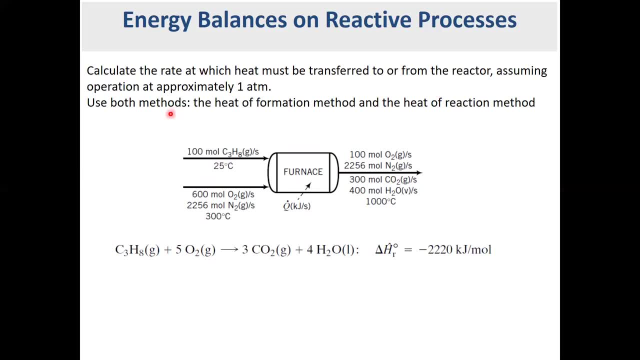 from the reactor, assuming of rate And operation is done, actually is happening at approximately one atmosphere. we want to use both heat of formation and heat of reaction. for sure, When the reaction- you see, when we have our reaction and the standard heat of reaction- is clear, we can use heat of. 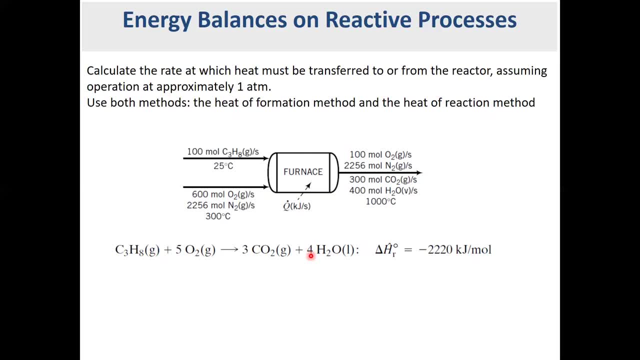 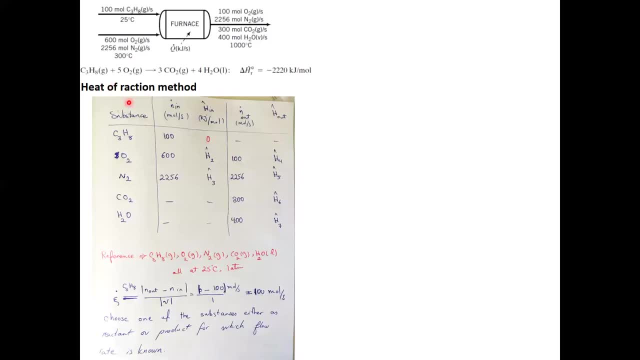 reaction method. It is easier method, but I actually use both method for you, conversely. So let's start. We want to use it from heat of reaction. So the first step I told you, provide the table. first of all, do all the material balance that you have in the system and then provide. 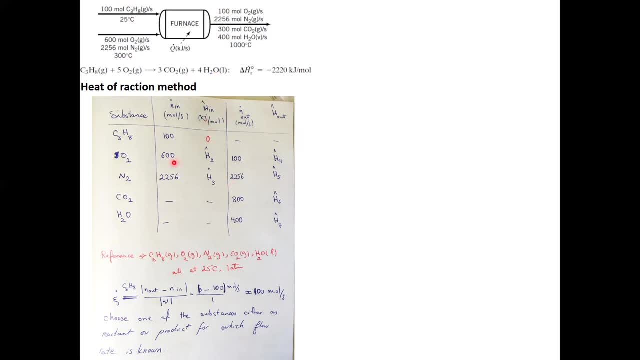 the inlet outlet enthalpy table right. So all the substance we have in this process We just list it down. we have here. So we list down a all the component involved in our process which is C 3, 8, 8 and C 3- 8, H 8. 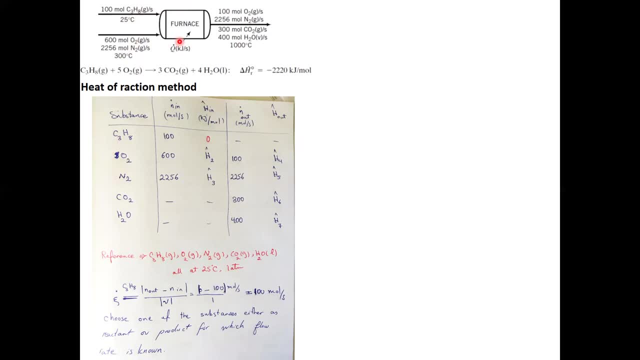 oxygen, nitrogen oxygen, nitrous water. so this is the component involved, all the component involved in our process. we just list them down. so these are the all information we have, all the component we have, what we know in the in. maybe all of them are not involved in the reaction, but anyway we. 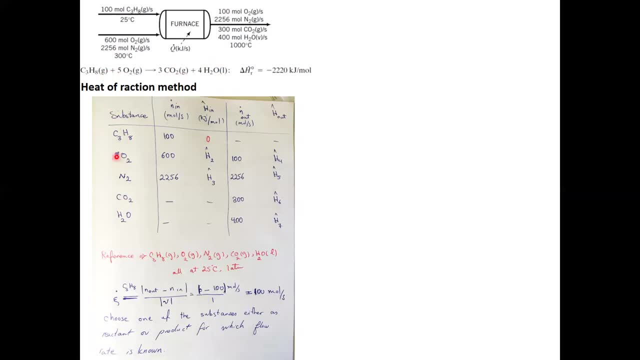 have to provide the information, all the substance we have. you have to list them in there, in that outfit, into application. so we have propane here, we have oxygen, have nitrogen, we have carbon dioxide, we have hydrogen. these are all the components involved, all the components involved, all the components involved in. 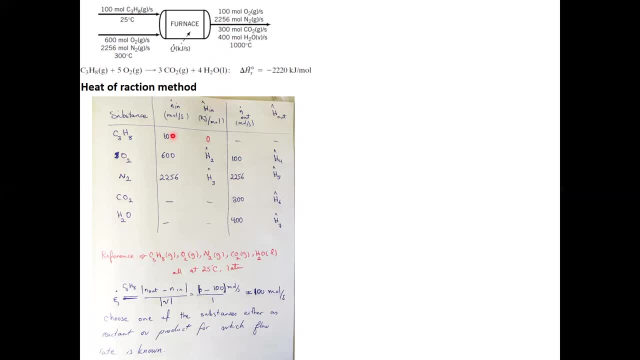 the component involved here. so, then, I provided all the information we have about material balance, so we have all of these clear for us. what is the molar flow rate more flow rate of each of the components? so we just substitute. these are the only three component involved in the inlet, the stream. that is why there 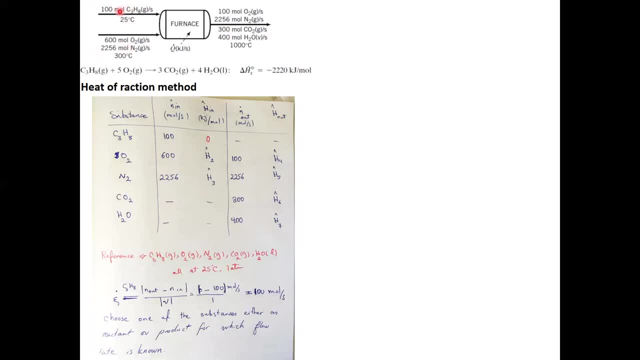 is no, there is, if you can see here. there is no oxygen, there is no, so sorry, there is no carbon dioxide, there is no water involved in the inlet stream, so I just put it dash without saying that there is no available in the output, the stream. we 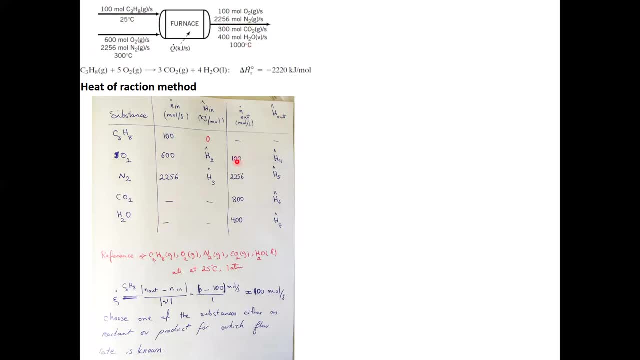 don't have any propane, but other components are involved. so we just consider those components. oxygen, nitrogen, carbon dioxide and water are all involved here. so we clearly know what is the temperature. a pressure is considered atmospheric from the problem is stated it is atmospheric pressure, so temperature is already clear for. so for each of this component, you know what. 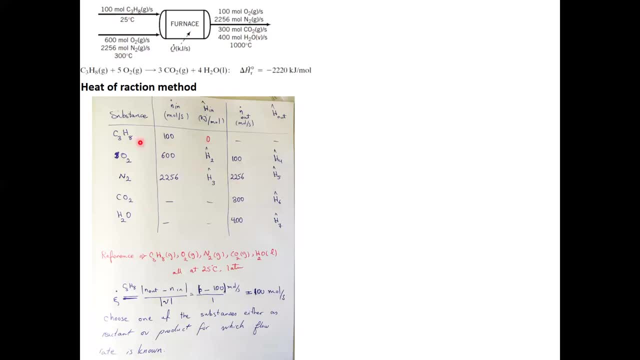 is the phase, what is the temperature, what is the pressure? so and actually we don't have propane in the output. that is why we didn't consider it's important to know how to provide. this table is very important. as long as we want to use heat of reaction method, we have to consider the. our reference is all the component. 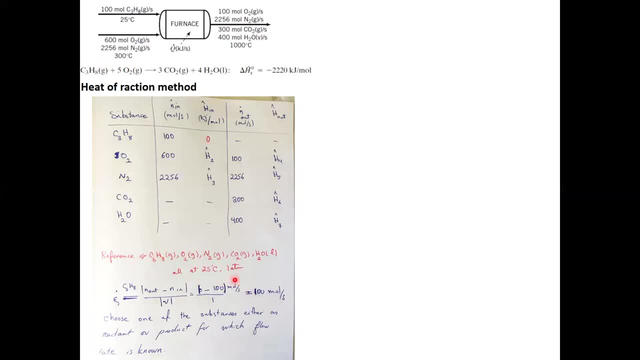 we have in this reaction at 25 degree one atmosphere at the phase. they are available in this temperature and pressure. we have some idea about some of the component at 25 degree and one atmosphere, like for example for propane. it is in gas form for oxygen, gas form for nitrogen gas. 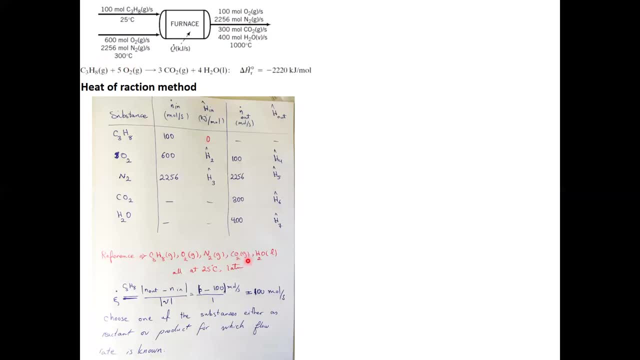 form for carbon dioxide. in this temperature and pressure they are all gas. but water, in this temperature and pressure, is liquid. so we have to consider our reference: at 20 degree, one atmosphere, the phase, what is the phase of heat, all the component that are involved in our process, at 25 and one. 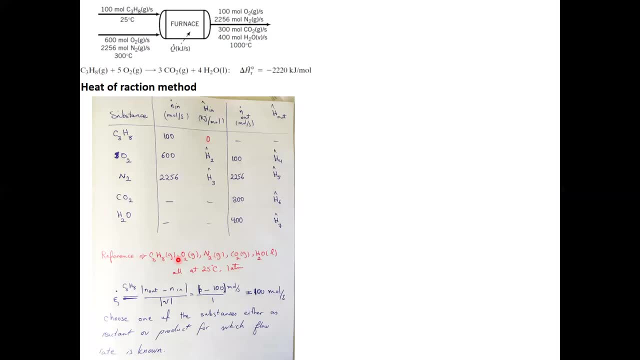 atmosphere. so it is not something we select by our self, it is something that existing in real situation at 25 degree and one as possible. so what you have to know exactly the phase, the temperature and pressure of the your reference point. so, referring to this reference point, we can see the only this is 25 degree 300. 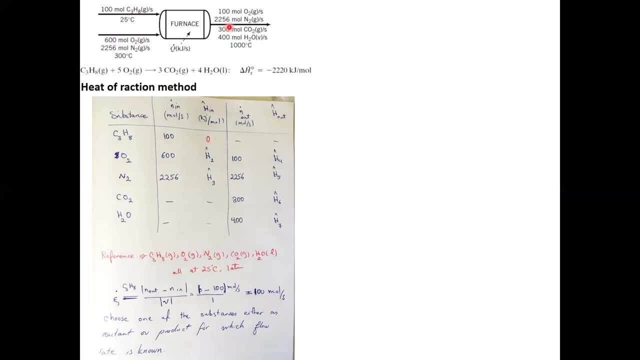 degree one at to the 1000 degree. the only component here that is in in this actually has the same temperature as the reference point is propane here, as long as this component is that in the same reference is existing at the same temperature of our reference point, we know for those. 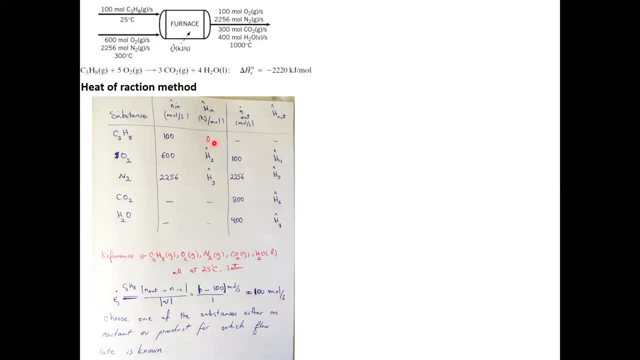 component at reference point. reference point is a zero in total, so that is why we put zero here. because, for a pain in the process, is actually available at 25 degree, which is out reference point. that is why we consider zero. the other are in different temperature, so we have to calculate the. 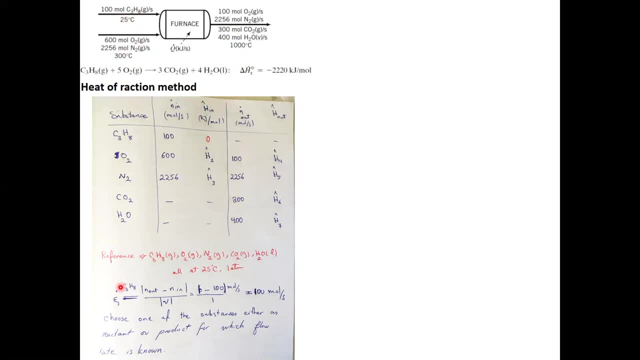 second point I asked you. the second is the next step that I have to consider. we have to calculate extent of reaction, so you can choose any of these components. I mean between propane, oxygen, carbon dioxide and water. you can use any of these components to calculate the loss of reaction between propane, oxygen, carbon dioxide and water. you can use any of these. 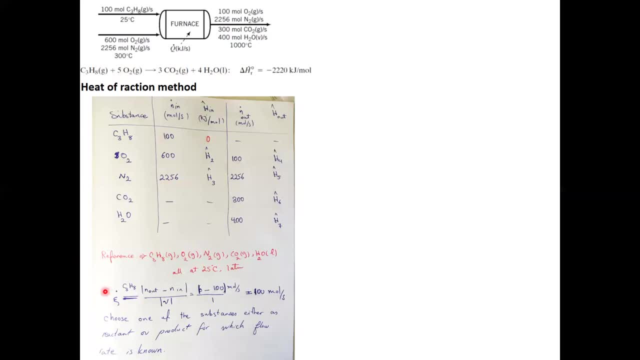 components of this four component and calculate extent of reaction, because both in that an outfit are clear. I'm just giving you example. I selected propane here. you don't have porophane in the outlet, so outlet is zero, inlet is 100, right. so divided by how much is the stoichiometric coefficient one, right so. 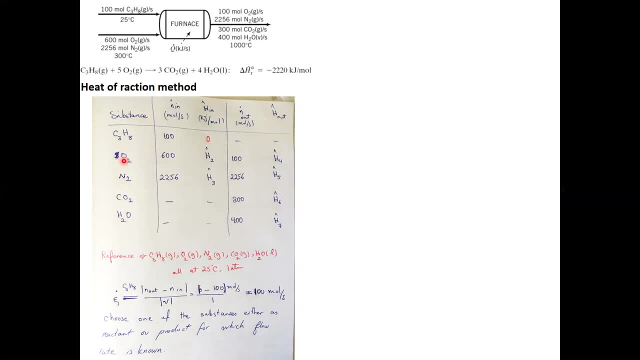 it is 100. okay, if you want to select oxygen, no issue. you have to mention: 100 minus 500 means 500 divided is two geometric a, a uh coefficient of oxygen, which is five. 500 divided by five is again 100.. so i mean that. 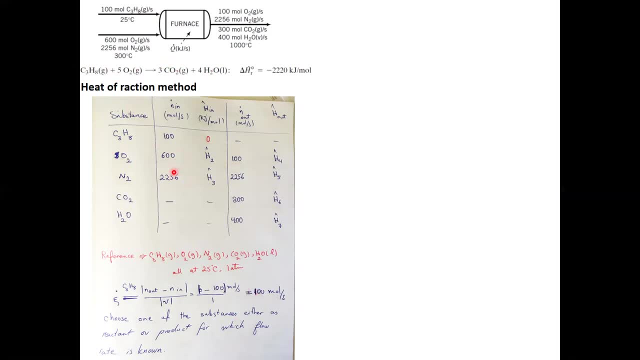 if you choose any of this component, as long as inlet and outlets uh mold rate is clear, you can calculate and you reach to the same value. so extent of the reaction can be calculated from either of these four components and they all should be same. so you can choose propane, like me. you can choose oxygen, you can choose co2, you can use. 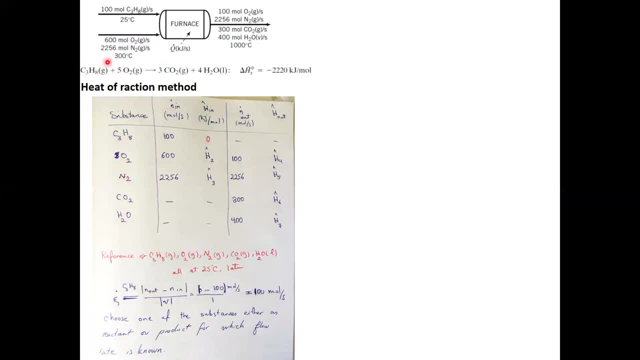 water. you cannot use nitrogen because nitrogen is not involved in this reaction. so it should be for sure one of the reactive components, either from reactant or from products. but you have to put it in the same equation and calculate extent of reaction. hope it's clear. so now we want to go to the next part. 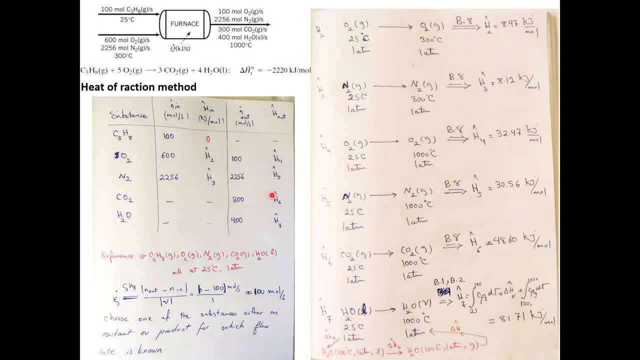 each of these specific entropy and calculate them. So we want to calculate H2.. H2 is oxygen at 300 degree, Oxygen 301 atmosphere. For all of them you have to consider the changes from reference point, as we discussed before. So you have. 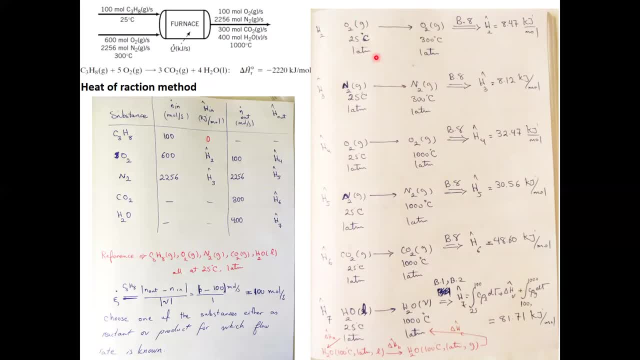 to consider. reference point is oxygen at 25 and water sphere, and final state is oxygen at 300 and 1 atmosphere. This is what we have as H2.. So for oxygen- this information you can refer to table B8 at the end of your book, The. 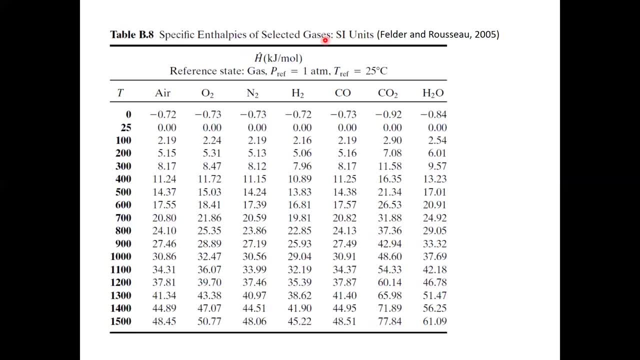 specific entropy of some gases is available in this table. You have to consider. if you want to use this table. your reference stage should be gas for all of this component. They are gas at 25 degree and one atmosphere right. So if your component is not gas, 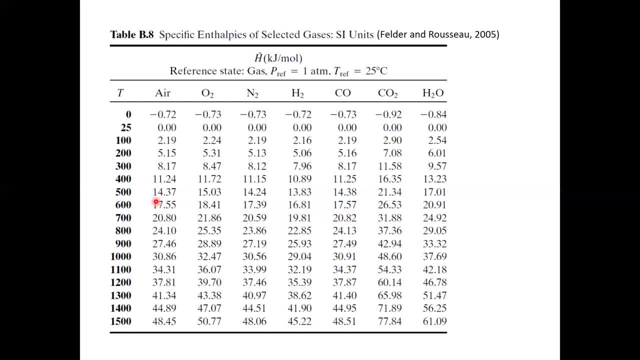 in this temperature and pressure, this table is not applicable. I think the only thing that you have to consider is water. You can use water only. you already considered this condition. I will explain to you. So this table is provided for you up to 1,500 degree. 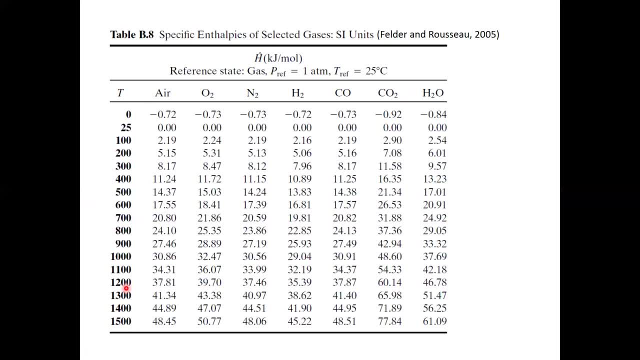 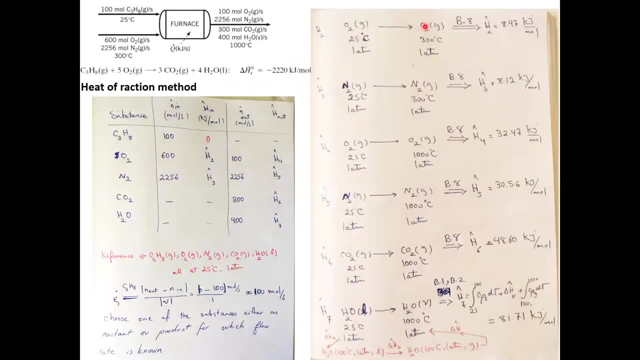 is given to you for sure. there are atmosphere, There are Celsius, because this 25 degree- and you see, at 25 degree it considered the specific entropy- is zero, because it is your reference point. So back to our calculation. we have, from this to here: 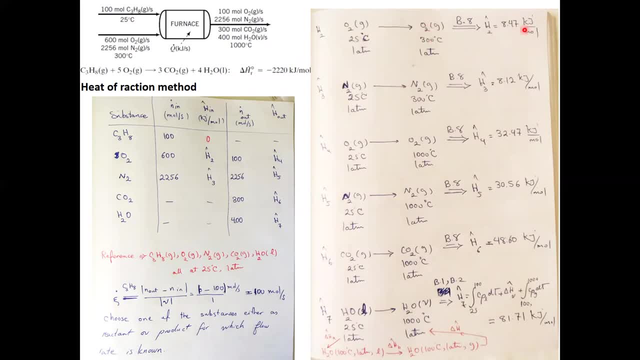 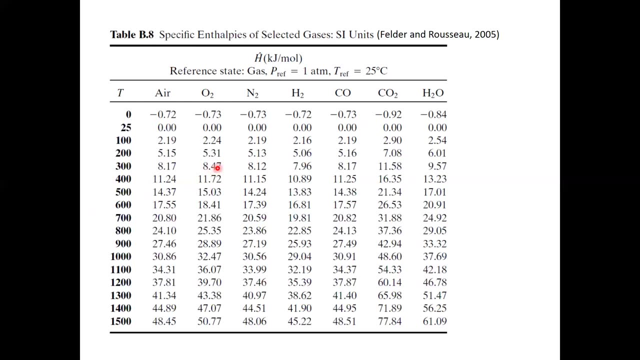 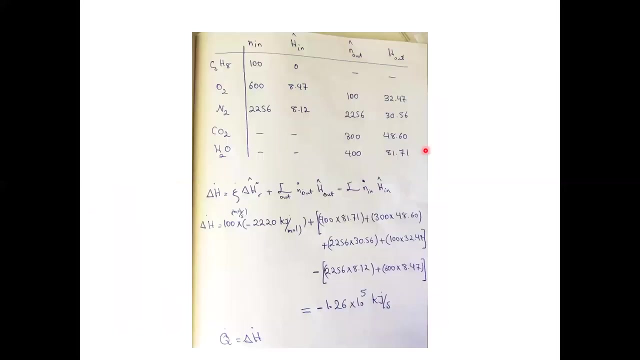 we know what is the specific entropy. We can read from the table for oxygen at 300. for oxygen at 300 is 8.79.. For nitrogen is 8.12.. For CO2, for water, for all of them is provided for you. 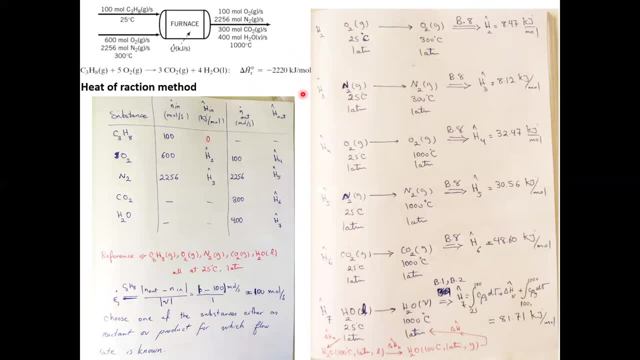 That is why that is how I read this value: H3 is nitrogen. H3 is nitrogen. What is the temperature here? 300 degree. Again, if we have the specific entropy from this reference point for nitrogen, we can use it. 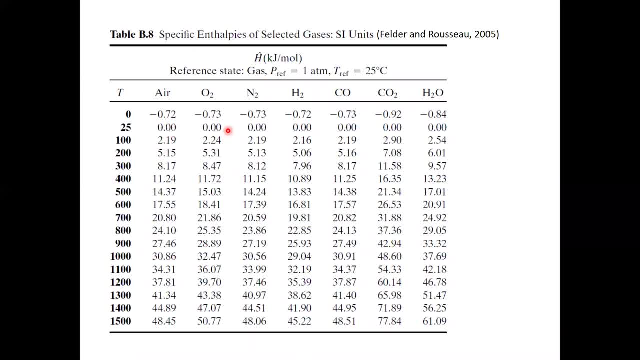 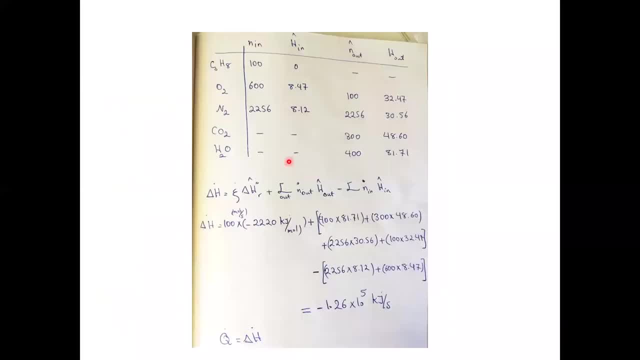 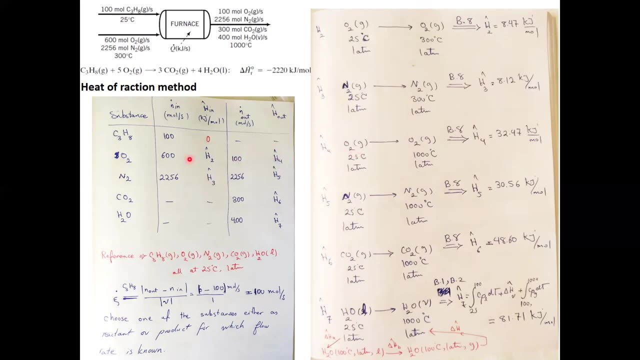 That is why in this table B8, you can go to 300 for nitrogen and read the specific entropy. So that is way I read it for now. H4,. H4 is outlet stream for oxygen outlet. What is the temperature? 1000. 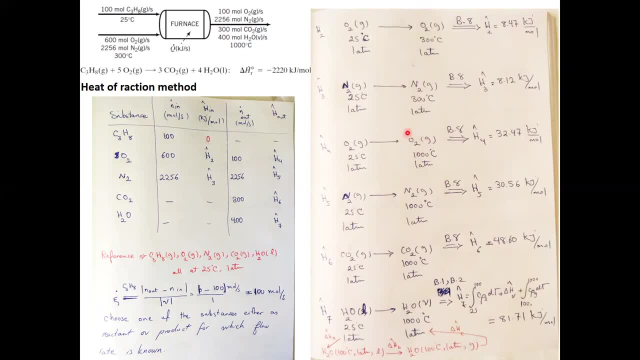 So here we have to read the specific entropy for oxygen and 1000 from the same table. Same goes to nitrogen, here H5, H6 and H7.. H5 is nitrogen, H6 is CO2.. There are these. all information are available in table B8. 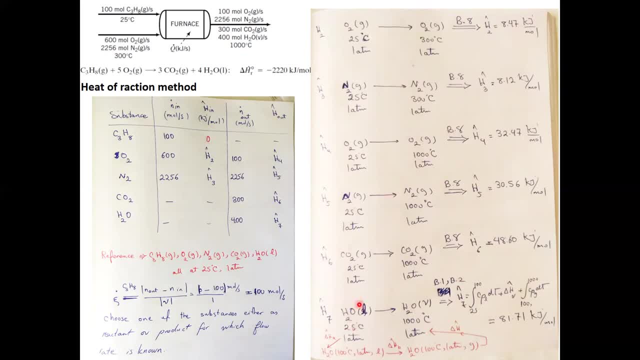 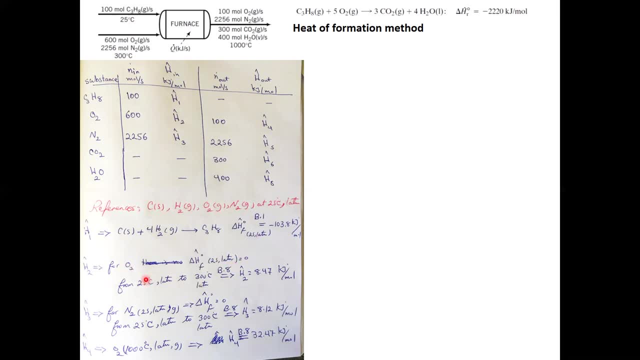 So for water, it is our reference point: water 25 degree 1.7.. So for water, it is our reference point: water 25 degree 1.7.. We have one more element. We have 2二, at least at the temperature of pressure. 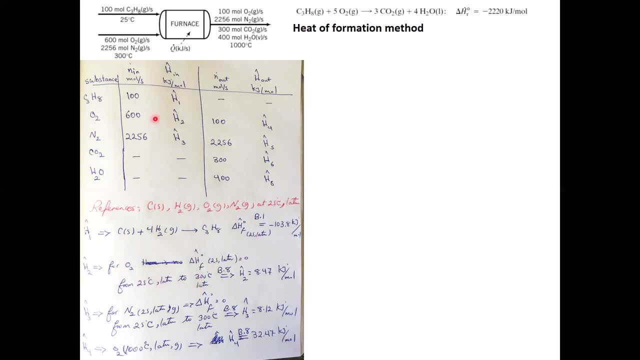 But what is the display, disrespectful to the distance between 2, the đi transmission signal around you and how you can send out temperature signals? By the way, we have the same thing with a surveyor unit. However, the temperature of pressure is not as a specified noise level as we do in the 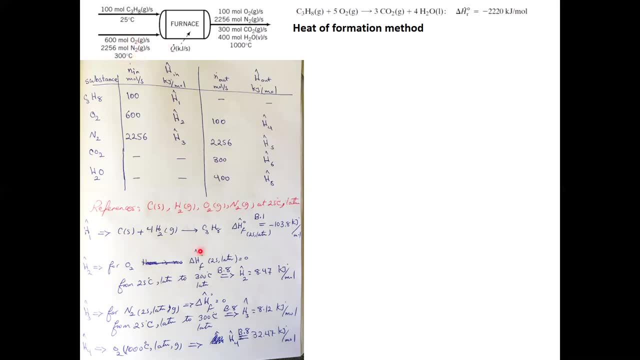 precular system. So if this air sample isiviable as Oxygen o2, at this temperature of pressure, But what is the specific enthalpy from 25 atm to 300, Kin-363est to 0,900, your reference. if it want to reach to 300, we have a table B8. We can go and 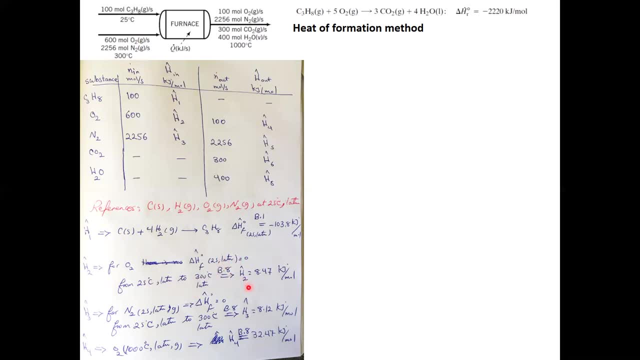 read what is the specific enthalpy of oxygen? to reach to 300.. The same thing goes to nitrogen. There is no heat of formation for nitrogen at 25 degree and 1 atmosphere, but to increase the temperature of nitrogen from 25 mm1 atmosphere to 300 degree, which is the temperature of the process you have. 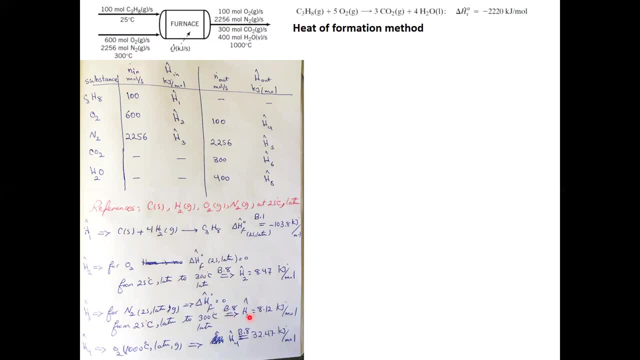 to go to table B8 and read the specific enthalpy of nitrogen at 300 degree. Again, in the outlet you have oxygen at 1000 degree. So there is no heat of formation for oxygen for 25 degree. but to reach to 1000 degree you need to read: 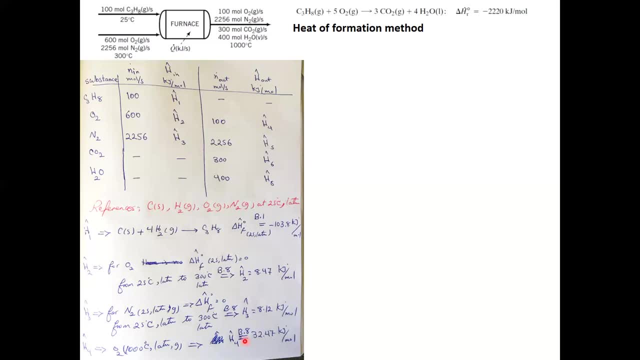 the specific heat of combustion, I mean the heat of the thermos. So if you change the temperature from 25 degree to 1000 degree from table B8. Now we reach to H5, again it's nitrogen at 1000,. so for nitrogen, 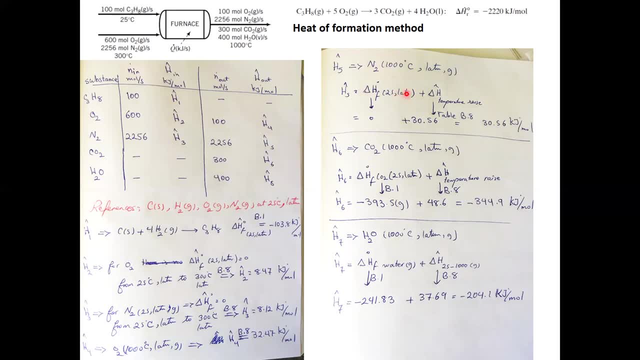 at 1000, 1 atmosphere. we know there is no heat of formation. but from 25 to 1000, we have to go to table. I just make it easier for you. We know delta H of formation should be read from table B1.. 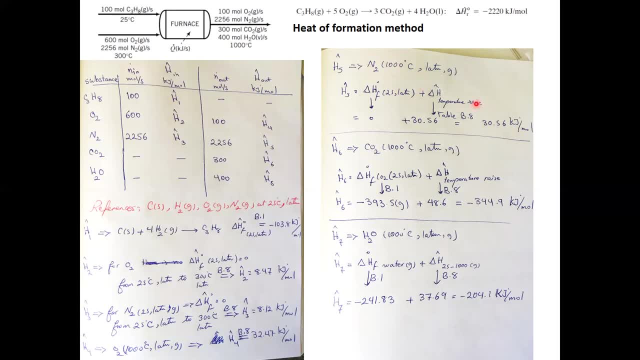 this temperature raise has to be considered from other way For us. for nitrogen hydrogen, CO2,, COI, water at gas form from 25 degree to any other temperature, we can read it from table B8.. For nitrogen to reach to 1,000,: 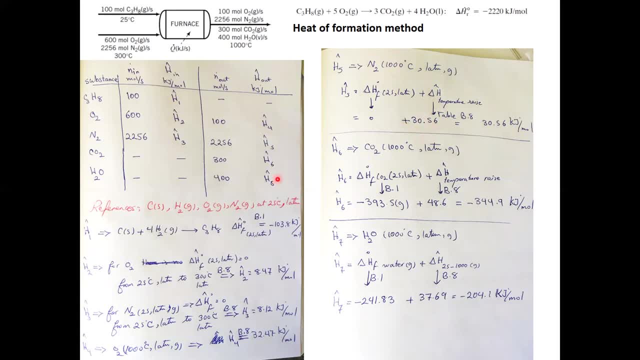 this value is available in table B8.. Now we reach to CO2 here. CO2 at 1,001 atmosphere and gas form is the process that we have. We have to consider first standard heat of formation of CO2 at 25 and 1 atmosphere. 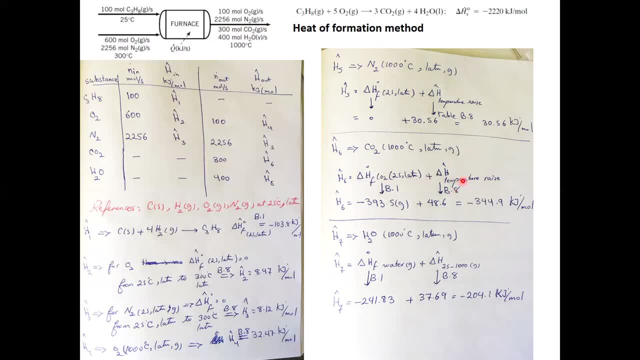 Then we consider how much energy we need to bring it to 1,000 degree. So we have to refer to the table B1 and read what is the heat of formation of CO2 at 25 and 1 atmosphere, which I read: 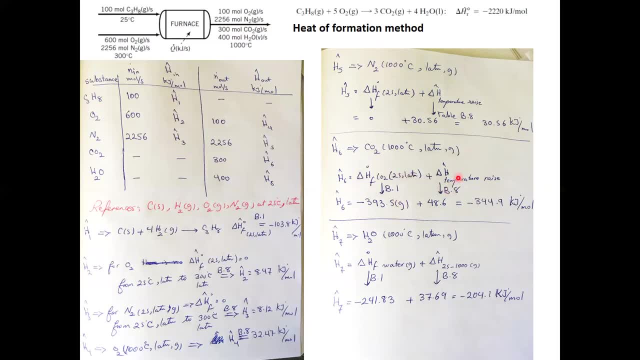 And then the table B8 and see for increasing the temperature of the CO2 from 25,. that means CO2 at 25 and 1 atmosphere, which I read. And then the table B8 and see for increasing the temperature of the CO2 from 25,. that means: CO2 at 25 and 1 atmosphere, which I read, And then the table B8 and see for increasing the temperature of the CO2 from 25 and 1 atmosphere. read up to here to 1,000,. read up to here to 1,000. 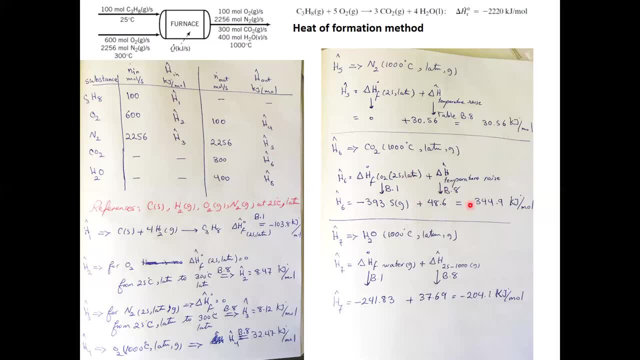 we can read this value from table B8. And we calculate the total amount of that specific energy for CO2 at 1,000 degree. and the last one is water. So we meat water at 1,001 atmosphere gas. So we meat water at 1,001 atmosphere gas. 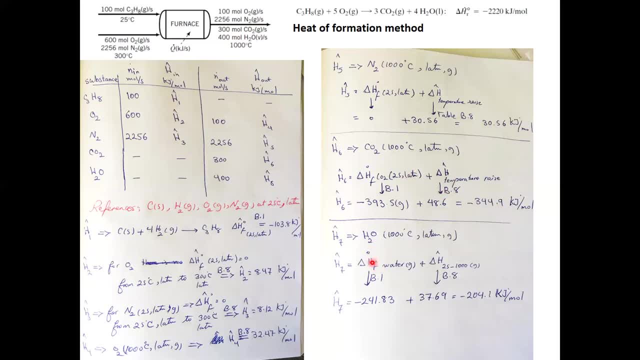 So first we have to consider what is the heat of formation of water. So you can consider. that is actually in the table B7.. B1. there is two types of heat of formation for water as gas, water as liquid. If we read water as gas from here to here, we can use table B8 because 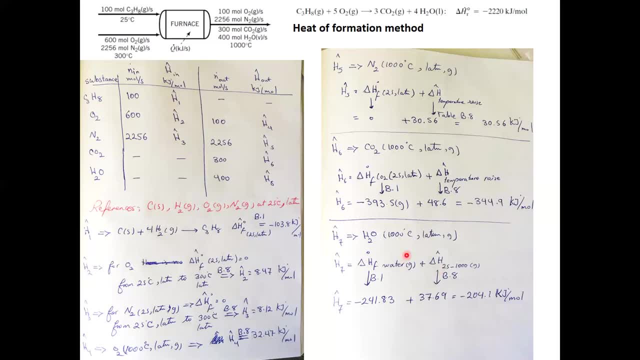 water as gas. if a standard is water gas, we can use table B8, but if it is liquid we cannot. So I read for me the standard heat of formation for water at gas form from table B1 for water and then use table B8 how to increase the. 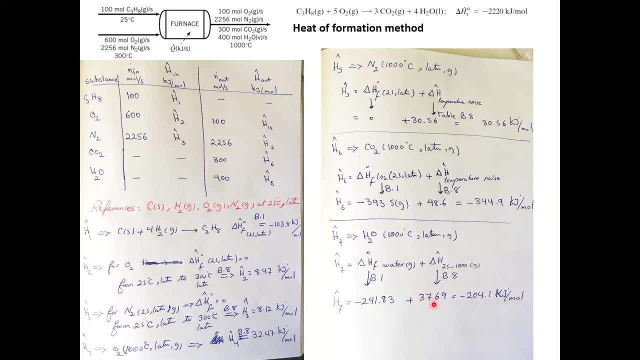 temperature of water to 1000 from table B8.. So it is not that much hard to calculate and to read most of them from the tables and data that we have. and I just read all the H that we want here, So the rest is easy, as you have all. 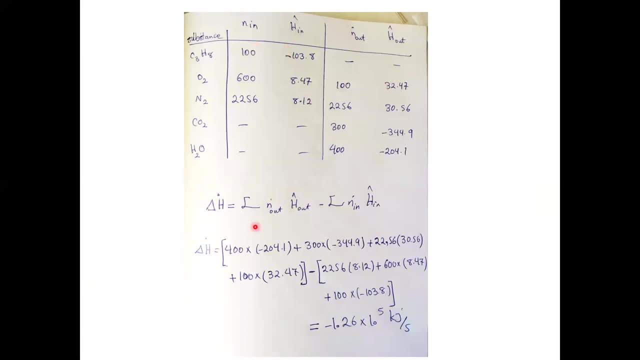 the values of H and N. you just have to put it here in this equation without needing to insert the heat of reaction. In fact it is already input, It's already inserted by the calculation. So I just put whatsoever, I just multiplied and add all this part in the 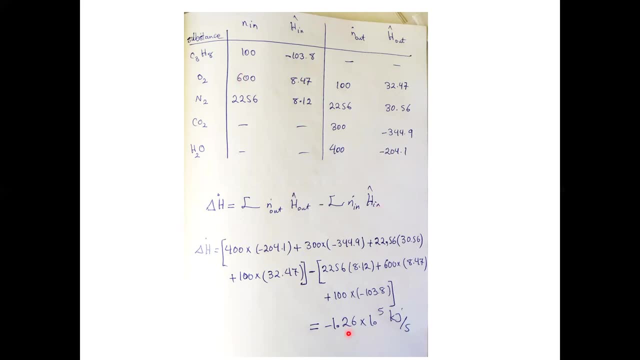 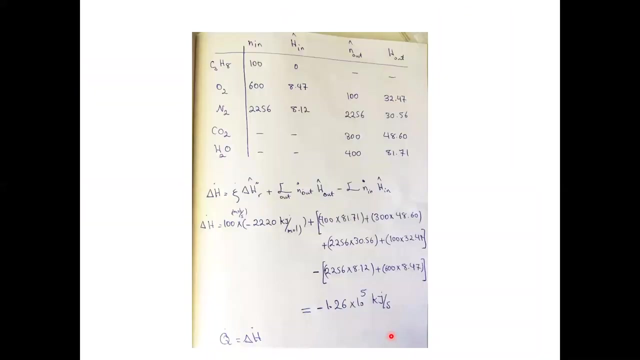 outlet minus the inlet part and calculated the rate of entropy change. If you compare this value- one minus, actually the minus one point two six multiplied by ten minus five, and minus one two six multiplied- you see the values are not that much different. so by using either, 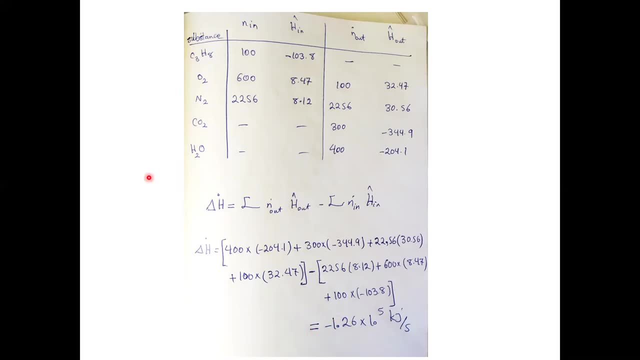 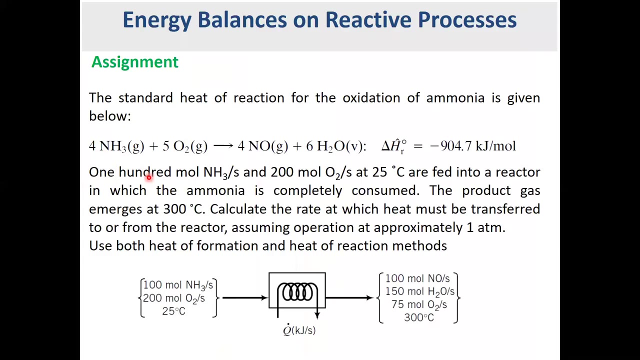 heat of formation method or heat of reaction method. values are not too much different, so you can use either of these two method to read it, to calculate the or to do energy balance on reactive process. I hope that you understand the main concept of this week of a study. please refer to the material and 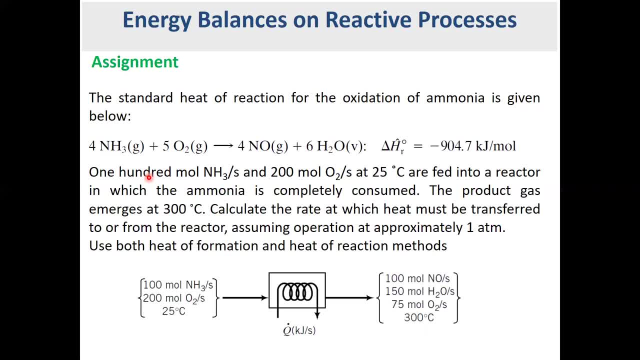 actually try to follow the step by yourself and calculate it and come to me if you have any problem or and then actually you need clarification. so I just provided one assignment for you here to actually try to learn what we have done so far on this problem. you can refer to your book to for more examples. 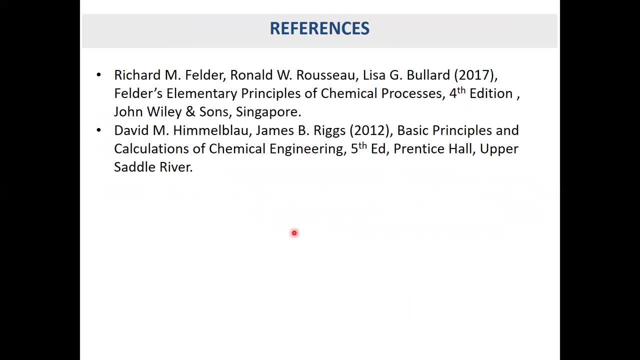 in history parts, and these are the reference that use in our material. I wish you all the best. have a great day, take care bye.